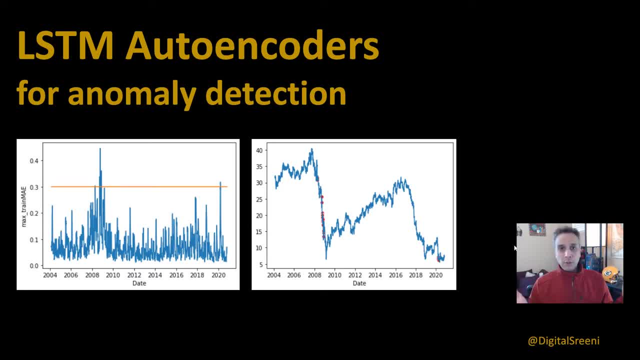 introduction and then we'll jump into the code and, of course, as usual, I'm going to share the code. so please watch the video and then download the code and do your things at your own pace. okay, And an autoencoder again in case you haven't watched my videos. just to quickly summarize: 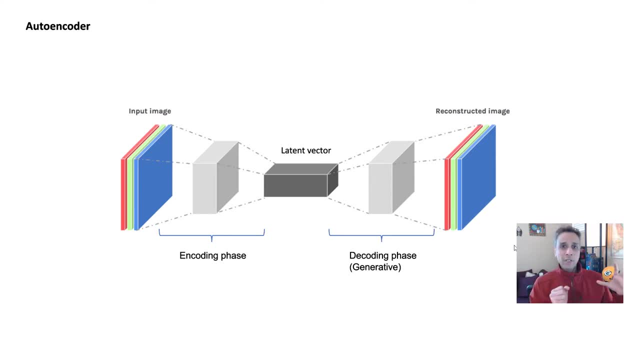 what is an autoencoder? It takes an input data that's bigger, let's say, and then encodes it into a smaller vector, okay. So, in other words, if you have an image like this, for example: okay, this image, let's say, the image is 512 by 512, okay, that image gets downscaled, okay. 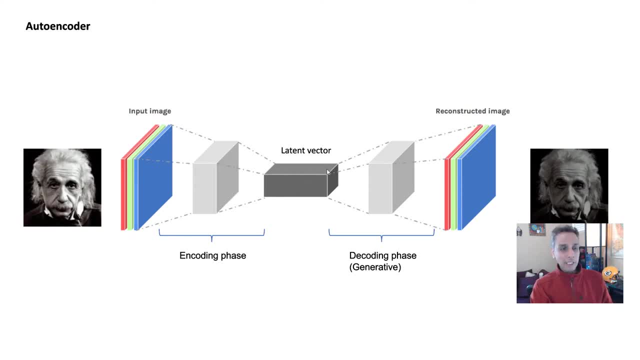 progressively, and then all the information contained in the image is captured as a latent vector or a vector. Let's say the vector has a dimensions of. in some cases it can even be like two. okay, Let's say the vector has a dimension of 10.. So 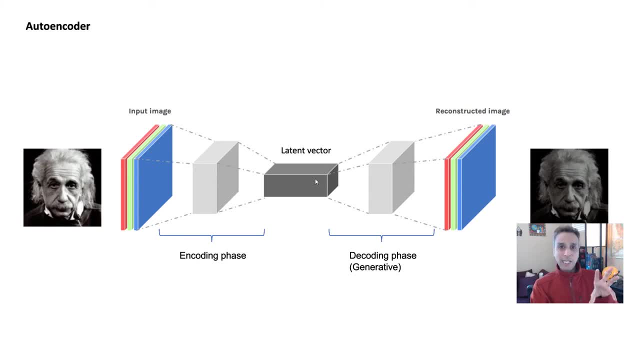 10 values or a vector with a dimension of 10 can capture all the information that's contained in this image, provided you know how to decode it right. This is where training is important. So you're training on the input image to get the same image back and you're adjusting the weights. 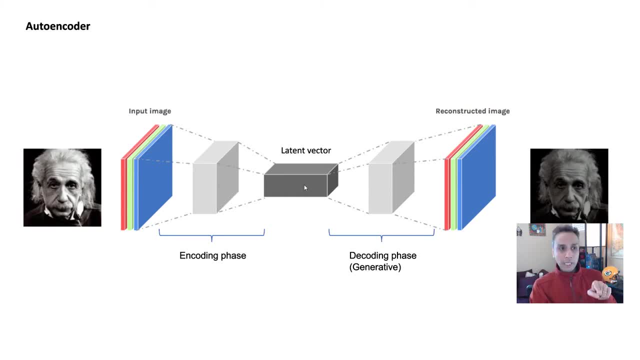 Why are you doing it? So you can encode the image into a vector and then use the trained weights for the decoder to decode that image back. Now, how are you doing this? When you're doing this, you're minimizing the reconstruction loss. 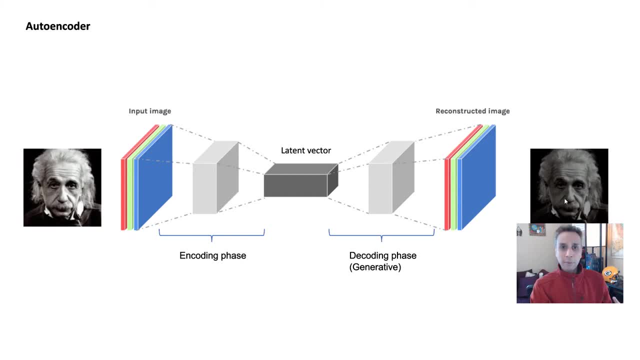 right. So if the output image is not as good as the input image, you're like: okay, train more, train more until you get the output image back, or as good as the output image is back. So this is basically what you're trying to do is minimizing the reconstruction loss. Remember that, because 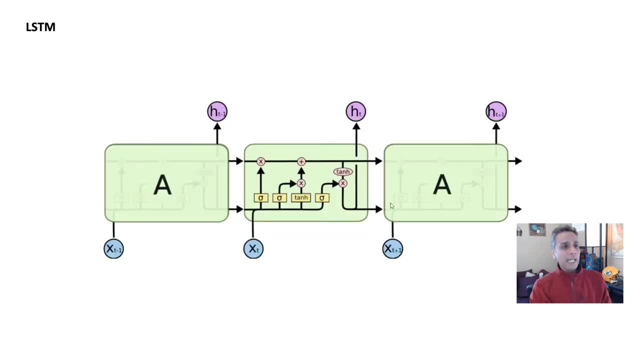 that's very important for anomaly. Now LSTM is again. I don't want to go through this entire structure because I made a full video on this topic. so LSTM has a structure that enables it to work well with time series type of data. So it only makes sense for us to build an auto-encoder using LSTM. 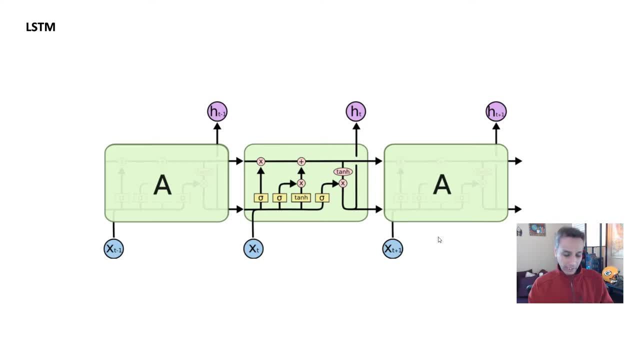 right For time series type of data. So that's the whole point here. So, instead of you know the you know, instead of basically using convolutional layers, let's say: right. so instead of you know the you know, instead of basically using convolutional layers, let's say: from the 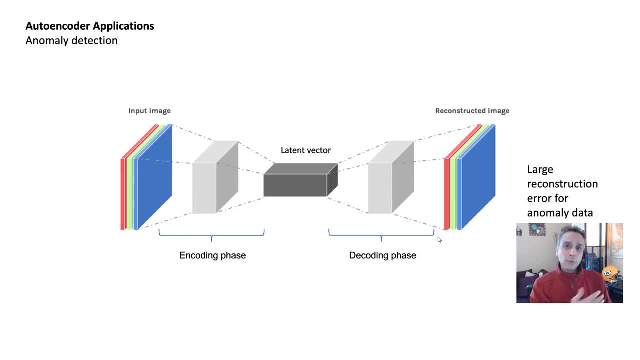 LSTM, right. So instead of you know from the LSTM, you know from the LSTM. you need to make an amazing structure. that's a lot more time-consuming and you can actually get the data out of the data layers. let's say, we can now use LSTM layers to put them together in an auto-encoder type of way. 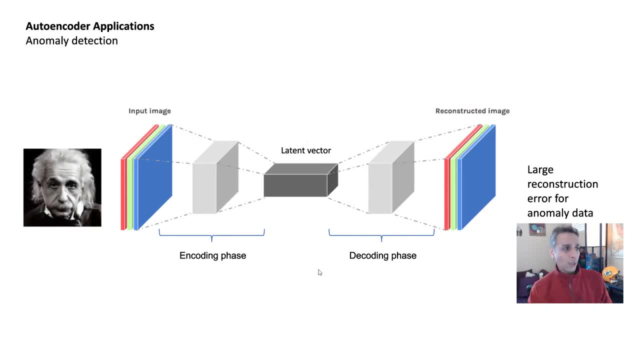 Now, how can we use it for anomaly detection? Okay, so our input image goes in. but then once you train it, you look at for the new data that's coming in. you look at the reconstruction loss, okay, And if the reconstruction loss is within the acceptable limits, then we say that okay. 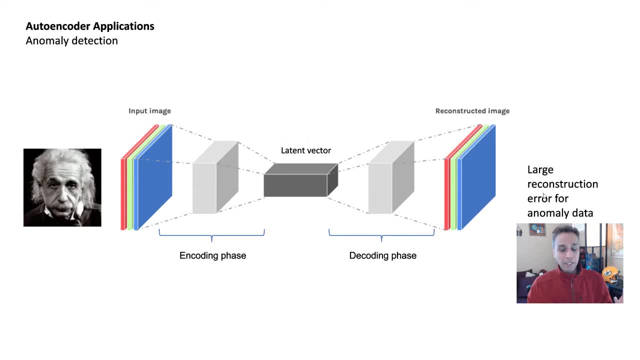 this is accepted, this is not anomaly. but if it's beyond that, this is anomaly, okay. So again, I think once we get into the code, it probably makes even more sense. but how do we do this with LSTM? Like I just mentioned, replace the convolutional layers with LSTM. okay, So here is. 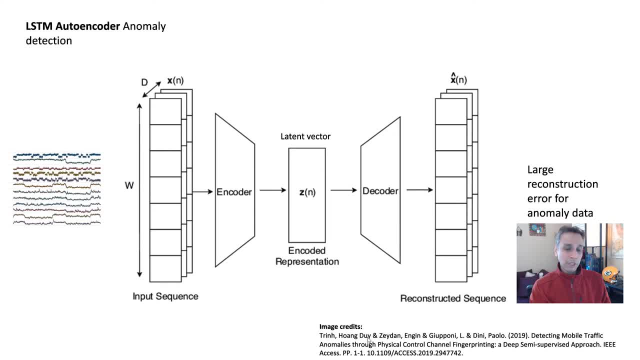 again a graphic and again the image credits. I just took this from a published paper right here, but this demonstrates it right. So here you have the input sequence and you have your LSTMs. Again it gets encoded. 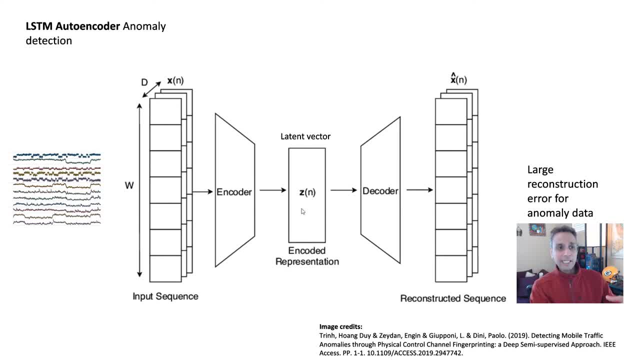 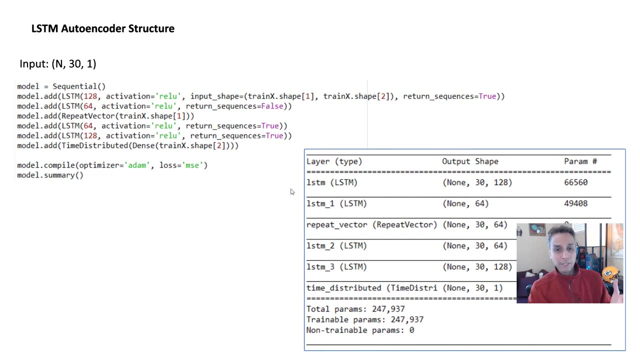 This data, whatever univariate, multivariate, whatever that data is- gets encoded into a latent vector and then you're decoding it. okay, I know this is at a very high level, so let's go in a little bit deeper here. okay, Some code. obviously you're here to learn about LSTMs and auto-encoders. 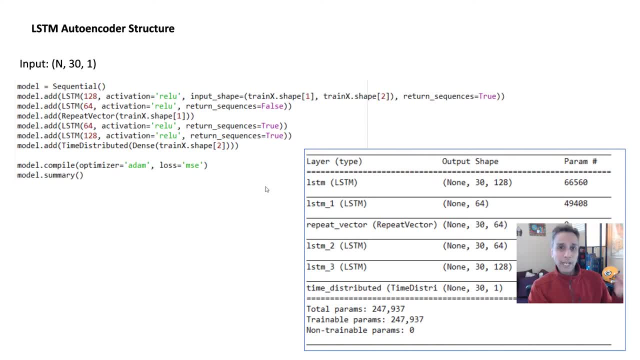 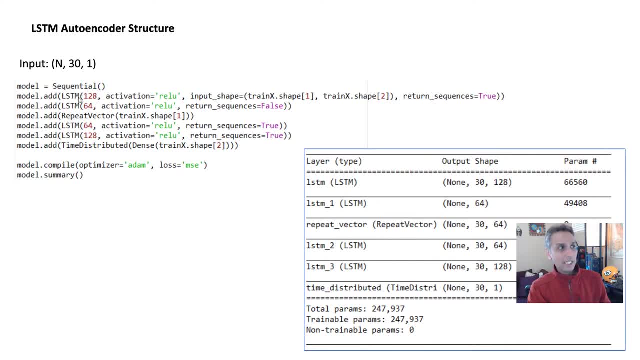 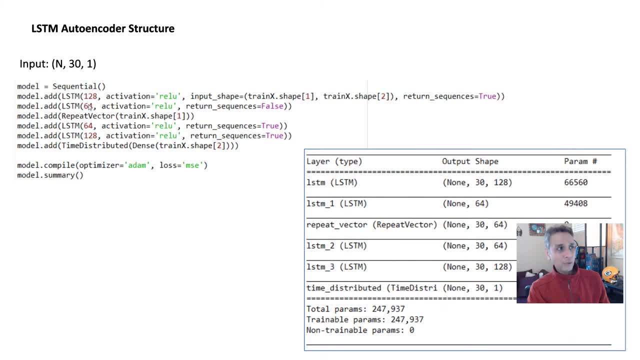 LSTM, layer 1, layer 2, here, 128 units 64 of these LSTMs. What that means is I have 128 of these LSTMs. okay, Units 64.. Now here, look at this. It says return sequences equals to true. I get to. 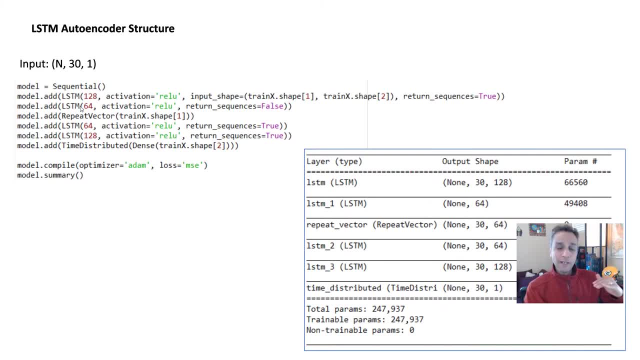 that in a minute. but if you really want to stack another LSTM, one after the other, you have to return the sequence, otherwise this doesn't have a sequence to work with. Okay, So you have to have a sequence Now. repeat vector is repeating this and you see how this is. 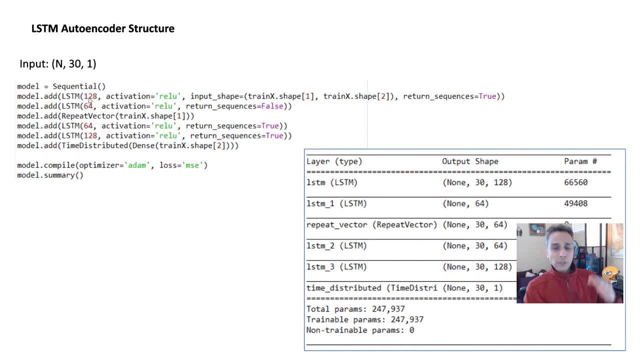 a mirror image. Now I have 64 and 128, okay, So I'm reconstructing it back. So this is the encoder part, this is the decoder part, and then we have the time distributed. I'll get to that in a minute. 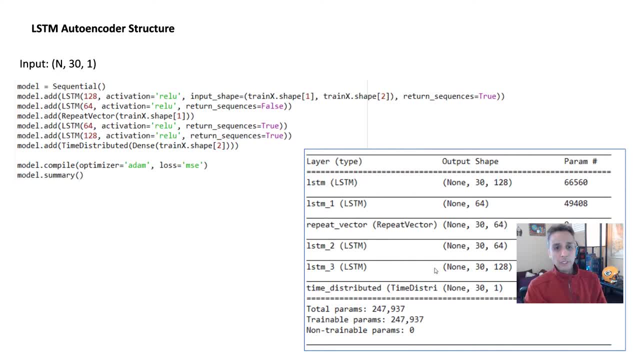 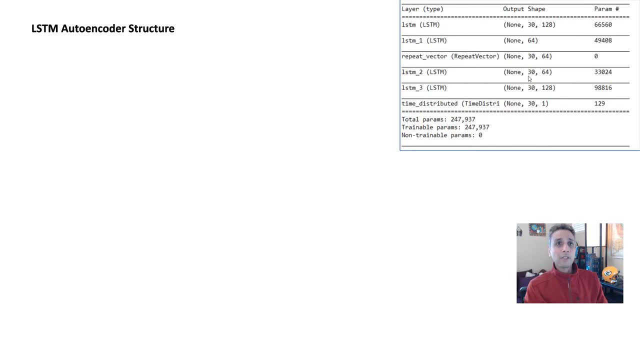 but here, when you print out the model like model summary, this is what it's going to print out. Okay, Now let's dig this one more level deep before getting into our code. I moved this up here so we can kind of go ahead and look at some of the text I put here. 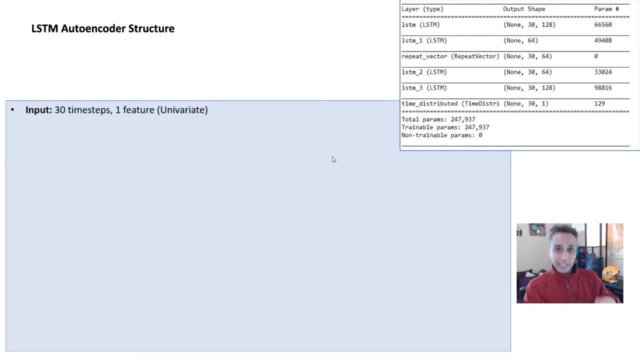 First of all, in the example I'm going to use right now, I divided the data into 30 time steps- okay, And one feature. That's it, okay, I have only one time series, okay, So 30 time steps and one. 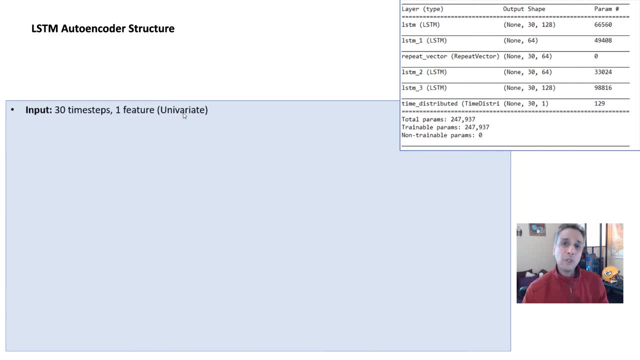 feature. Let's look at stock market data. In fact, we are going to look at GE stock index. so it's basically the closing. you know price for every day, So there's only one variable right now. okay, So 30 time steps. one feature: Now it goes into this layer one. 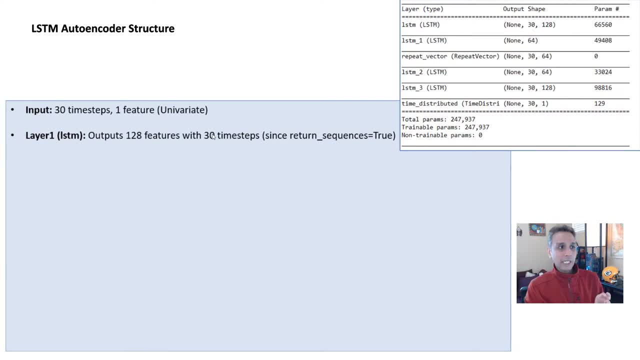 which outputs a shape of 30, because I have 30 time steps and then 128 features. okay, So it's returning 128 features And if you remember, we had return sequences equals to true. okay, So that's why it's returning us 128 of this. okay, And for each of the time steps, 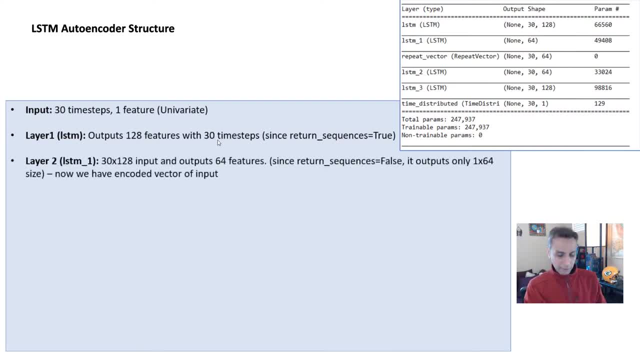 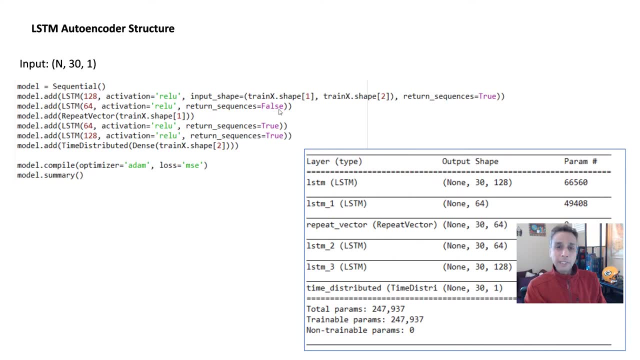 for 30 time steps And the next one, if you remember, we have return sequence equals to false. If I go back here, it says return sequence equals to false. right there, that means it's not going to return the sequence for all of those 30. So my shape in this case is: 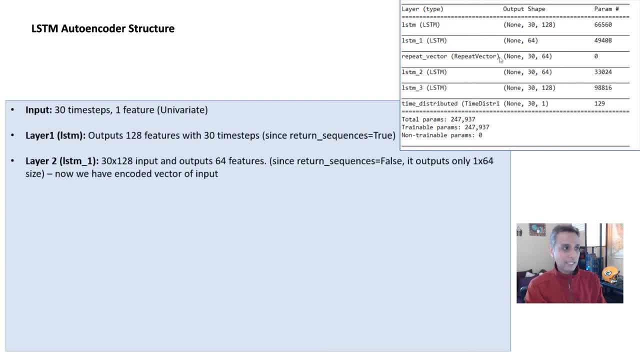 going to be only 64, okay. A vector of size 64, okay. So input for this layer, 30 by 128, and output is 64 features. And, like I mentioned, since this is false, it only returns one vector. 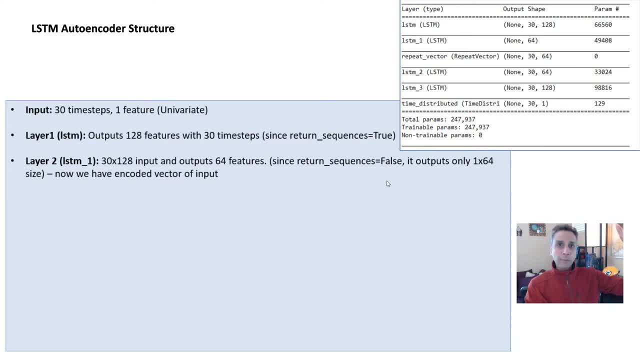 with a size of 64. This means we encoded our input, of whatever size okay, into 1 by 64. This is our encoded value. Now it goes into this layer, one which outputs a shape of 64. So that's. 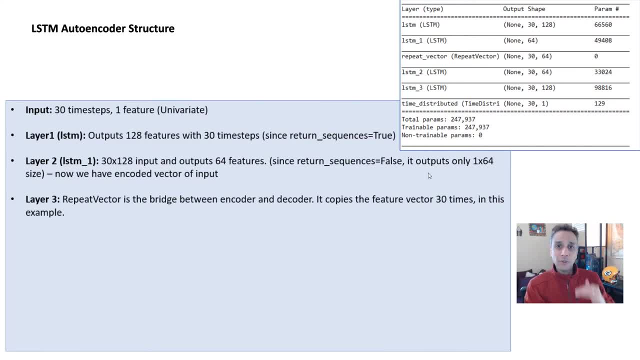 something called repeat vector. This repeat vector is the bridge between encoder and decoder for an LSTM time series in autoencoder, And what it does is it copies the feature 30 times. So now we have 1 by 64. It just copies it 30 times. It repeats it 30 times. That's why it's called repeat. 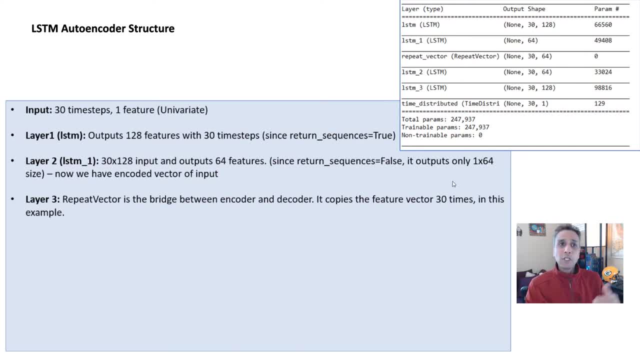 vector okay. Why does it repeat by 30 times? Because when you go to the next layer- LSTM 2, you need 30 by 64.. So it copies it and then it supplies that as input to the next level. 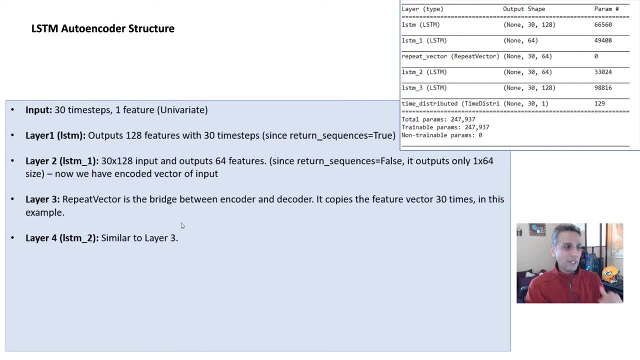 So that's why you have LSTM 4.. There's no tricks here. This is very similar to layer 3, except we're going in the opposite direction, right? So here, 64,. LSTM 3,, which is our layer 5, is also similar to the other layer. 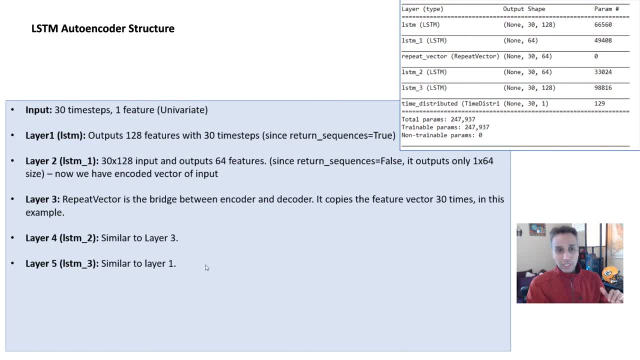 which we already have to layer 1.. So no tricks here, okay, And finally the time distributed. right here you see, the dimension of this time distributed is basically 30 by 1.. So what this time distributed does is it creates a vector internally. So what's going into our layer? 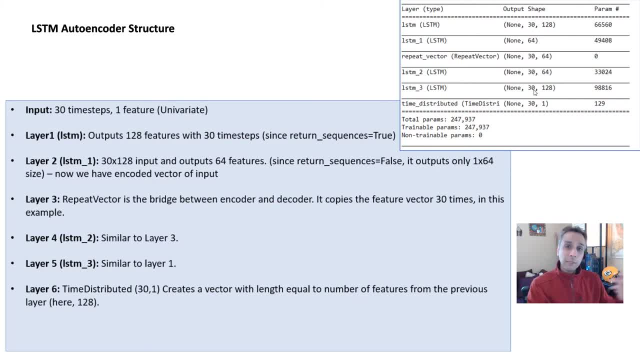 6? What's going into our time distributed, A output of size 30 by 128 is going in. right, It goes. 30 by 128 goes in And it creates a vector with length equal to the number of features from previous layer. How many features do we have? 128.. It creates a vector of 128.. What happens is: 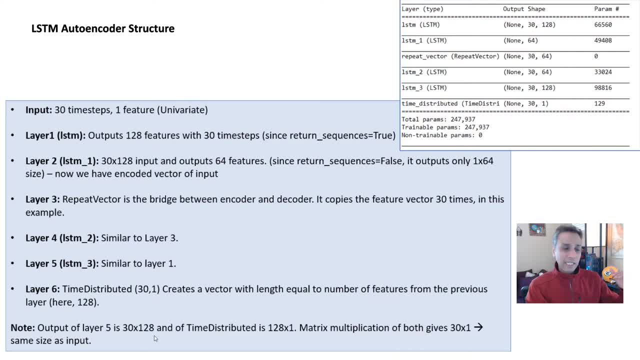 previously. here you have 30 by 128, and the time distributed is creating a vector of 128 by 1, right, It creates 128.. So when you do matrix multiplication of these two, you get 30 by 128 times 128 by 1.. You get an output of 30 by 1, which is nothing but our input. 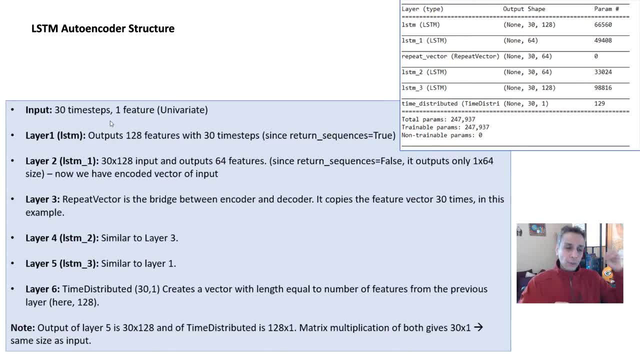 dimension. So this is our autoencoder. You start with some size, you go down to the encoded- whatever that encoded value is, you know vector is- and then you're decoding it back. So during this process, obviously you have a loss function and you're training this. 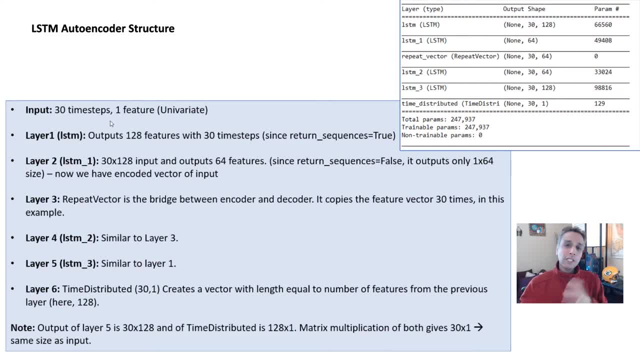 And once it's trained, now you know what the reconstruction loss is. Now you put new data through it And you can see that you have a loss function. and you can see that you have a loss function and just look at the reconstruction loss. okay, if it's above certain threshold. 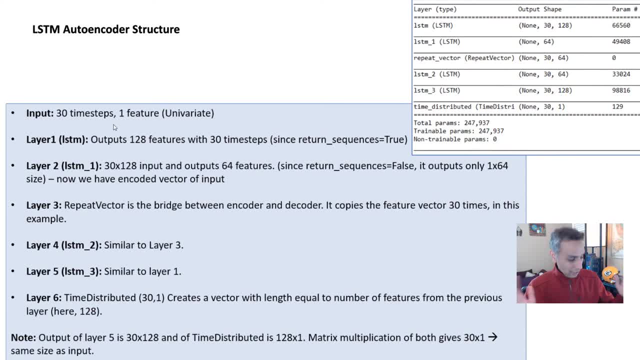 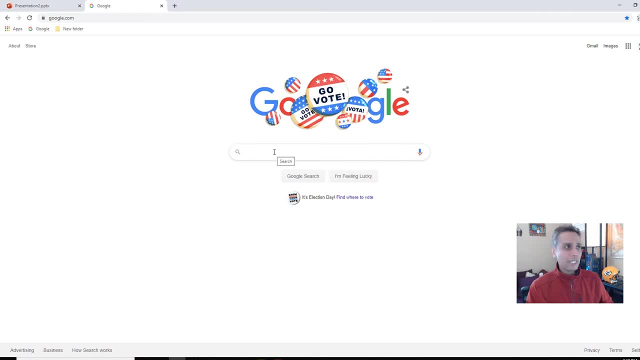 then, well, you have an anomaly. that's pretty much it. now let's jump into the code. hopefully this makes sense. okay, now let's jump into the code. and, by the way, the data set I'm going to use is GE. what's the best way to do? GE stock I? 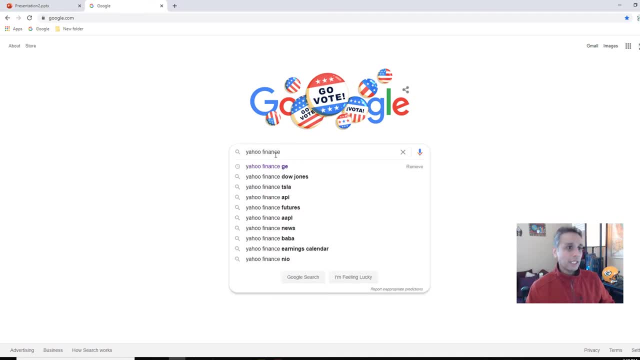 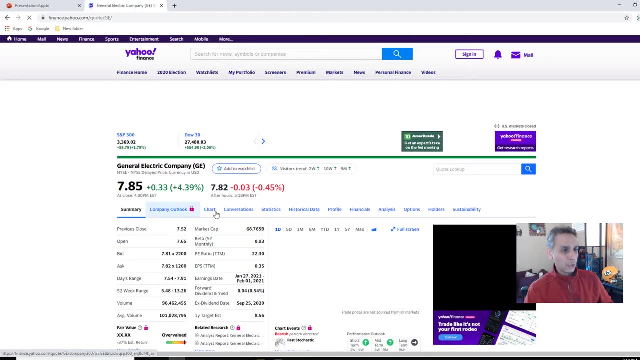 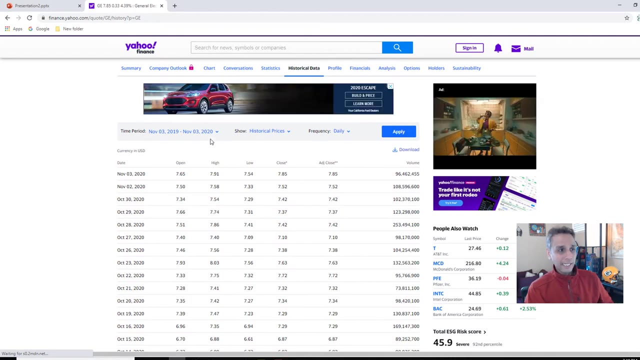 think it's Yahoo Finance and GE. as you can see, I searched for this before Yahoo Finance, GE, General Electric and you can go to historical data and you can select your start date and end date, whatever the end date is- right now it's November 3rd 2020 is the end date that's selected here, and you can go ahead and download. 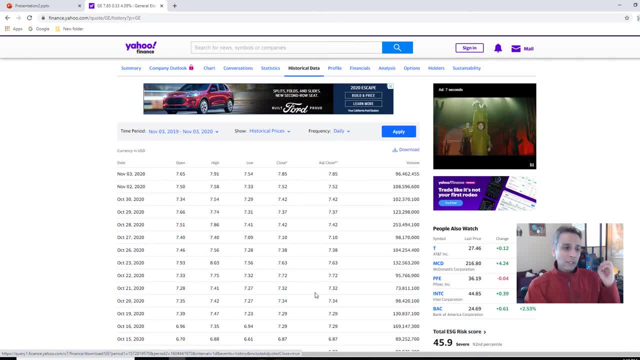 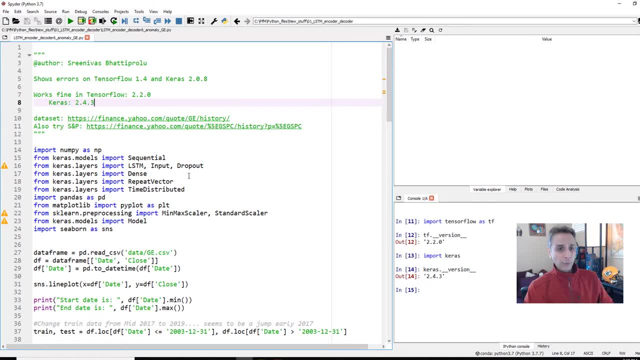 it and it downloads a CSV file and you're all set, okay. so that's exactly what I'm going to use in our video today. okay, now one other note. as you can see, the tensorflow version that I'm working on is 2.2.0 and Keras is 2.4.3, and it's very normally. I don't even mention about this. 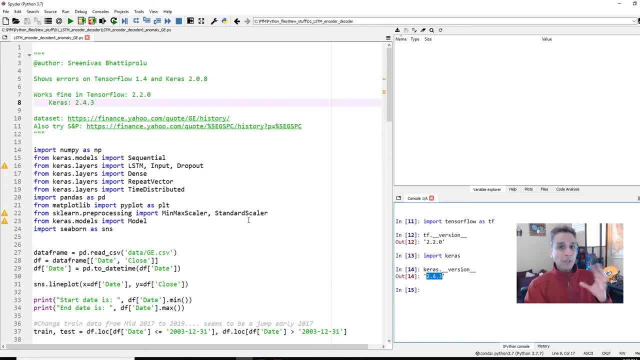 because things work on all tensorflow versions. one point something, two point something for the code that I test. but in this example it's not gonna work on tensorflow 1.4 and Keras 2.0.8, possibly because of this time distributed and repeat vector. maybe they're not available. I didn't dig too much into. 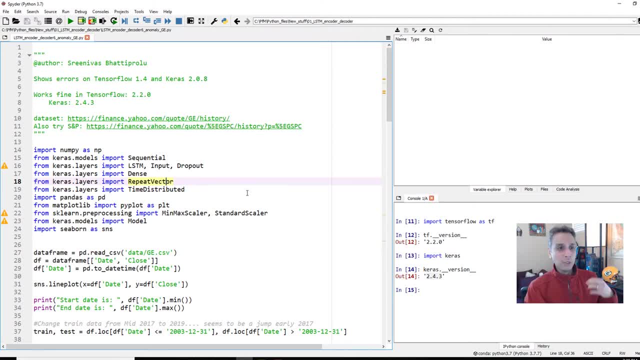 this. it gave it through some error and then I changed my environment to Python 3.7 with these two. okay, I should have investigated this, but again, the video is not about that. okay, and I assume most of you are working on latest versions anyway and this works. 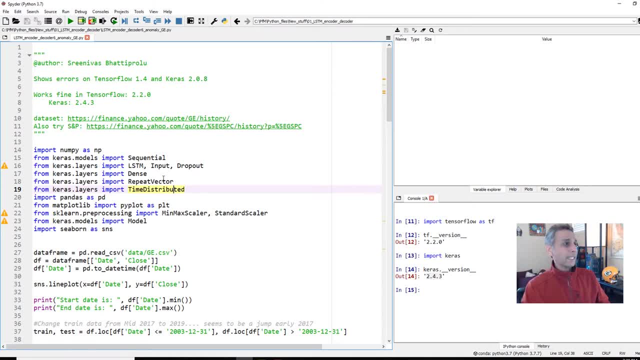 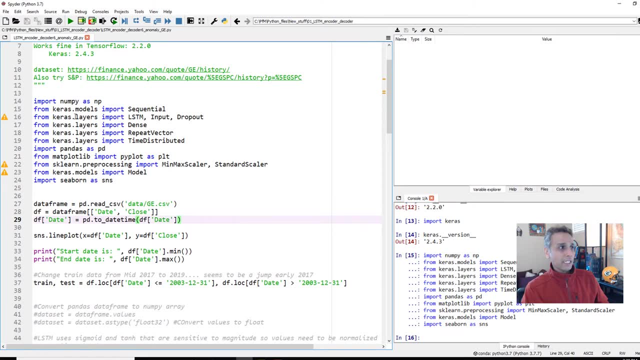 great on Google Colab, okay, okay. now let's get down to this. what do we have? let's have run all of these libraries again. this is basically Keraslayers. we are importing LSTM: input, dropout, dense, repeat, vector, time distributed. I should have just imported all of this in one single line, but anyway, I hope you. 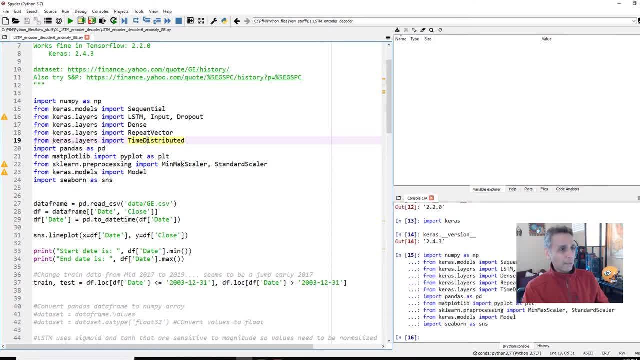 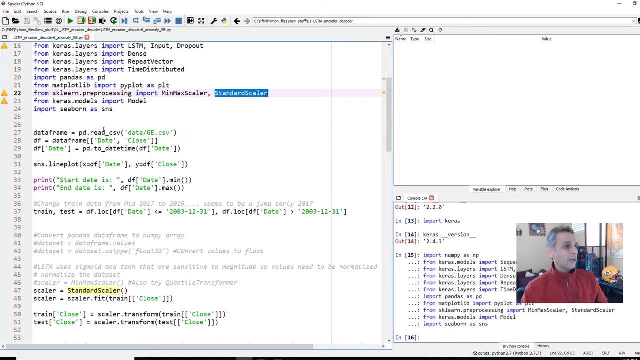 know what's going on here, and we are importing both min max and standard scalar. I think I ended up using standard scalar instead of min max, but I usually import these and then decide which ones to use, so you're probably a bit more organized than I am, okay, so now let's get our data. so I downloaded this into a. 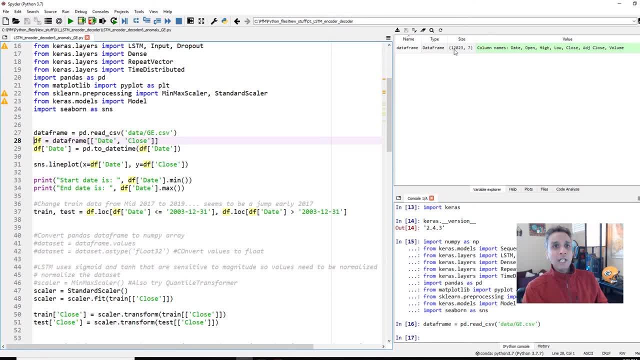 CSV. so I'm gonna just go ahead and read that. you can see I have 12,000 823 rows and 7 columns. and what columns do we have? I think it makes sense to have a quick look if it opens here. yeah, so we have date. okay, starting from 1970, that's. 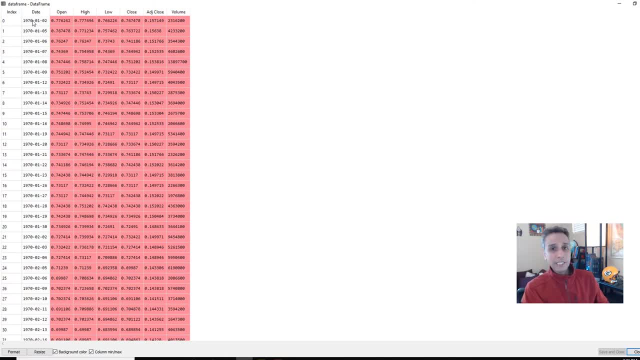 what I downloaded. you can download it based on whatever you need. GE is a very old company, so I think it goes back to the first few decades of the 20th century when it comes to stock market. okay, so we have the open value, high for that day, low close and then volume, and all that. so let's just focus on the. 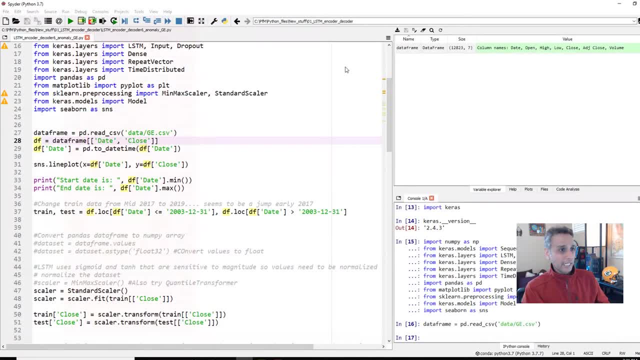 closing value, because that's basically what we're doing and it's based on the- the end of the day, the value of the stock. so in the next part, I'm creating a data frame with only the date and the closing value and, of course, now, if you look at this, the date is just in the object. 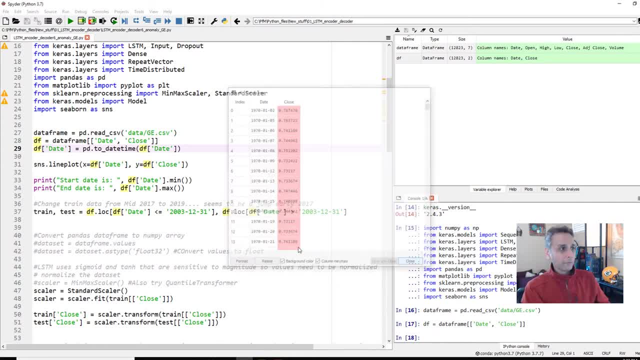 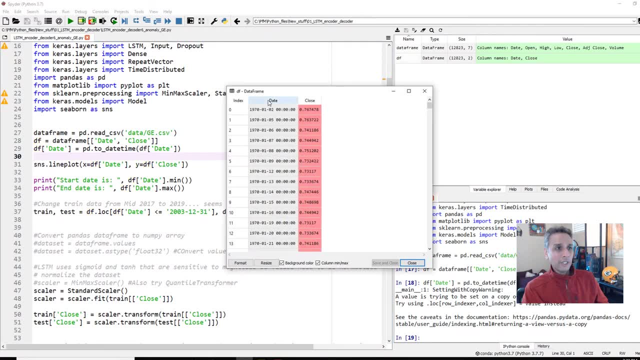 form, meaning it's not in the date time form. so let's convert that to date time format and when we do that, you can open it. and now you can see that this is in the date time form. so now it understands when I try to plot or use it, as you know, later on in the code. okay, so let's have a. 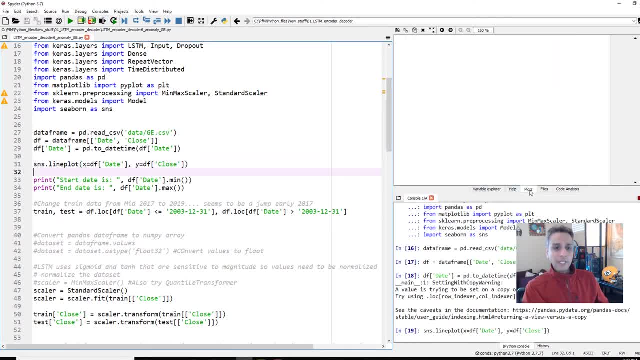 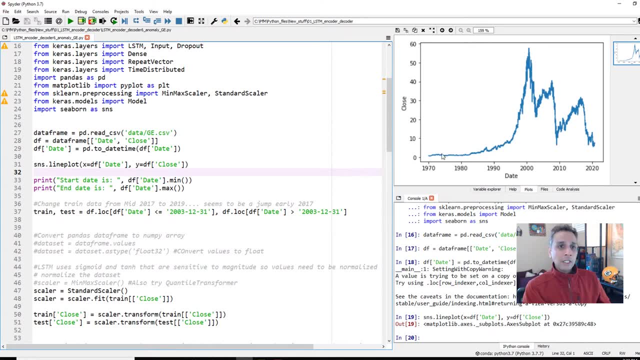 quick look at how it looks like. how does the stock look like? okay, so there you go. so 1970s. we should have bought a whole bunch of stock back then, but I was just a baby back then, so, huh, and most of you probably not even born, and it's a. it saw its best days during early 2000s and later on now. 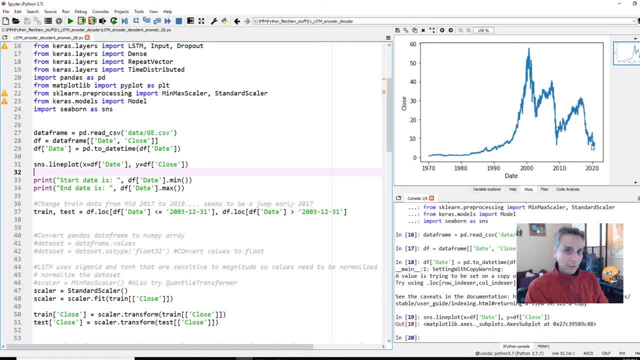 you In 2020, its it's back down to below 10 dollars. maybe it's a good time to purchase it if you're interested in investing it in this for the next few decades and if you believe in the direction that this company is going okay. so enough of that. let's go ahead and print the start and end date. so, as you can see, 1970: January 2nd because January 1st- obviously stock market is closed on January 1st, and then the end date is October 29th, 2020. okay, so I just chose to delete some of the later dates. 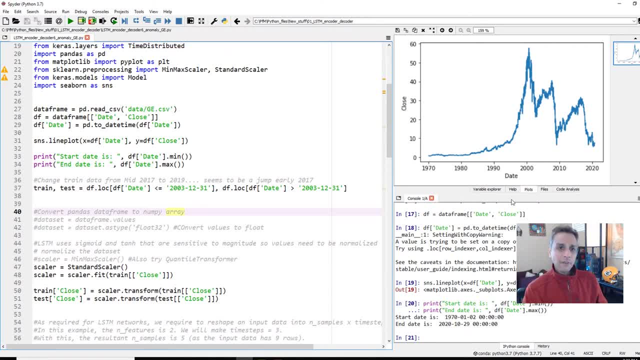 okay, now for any, for any of this data sets. we always divide this into train and testing, right? so for a typical time series, we actually said: okay, let's take 70% or 65% as the training and remaining, you know whatever, 30% or 35% as testing. 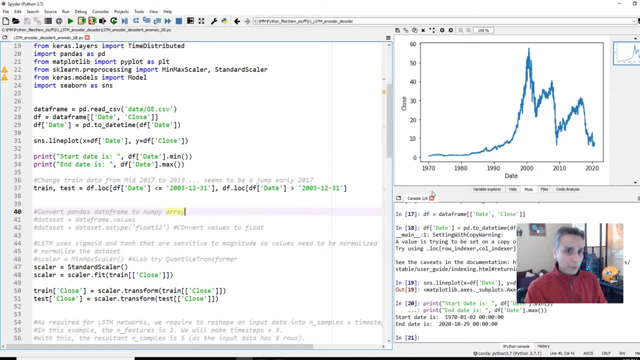 but in this case I'm actually defining this as up to. I looked at this and I'm like, okay, what is the best one? do I want my model to be trained on these Peaks and all of this stuff? I think, why not? yeah, so I just took up to 2003 somewhere. 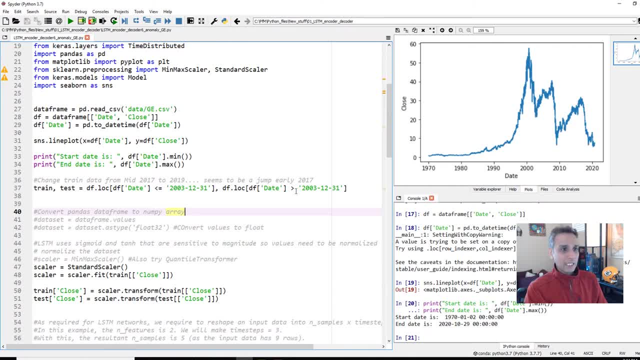 around here up to this point, as the training and the testing is everything after that, I'm going to use it for testing. okay, it's up to you. you can pick any other stock or you can even look at the S&P index. it's up to you, but I'll. 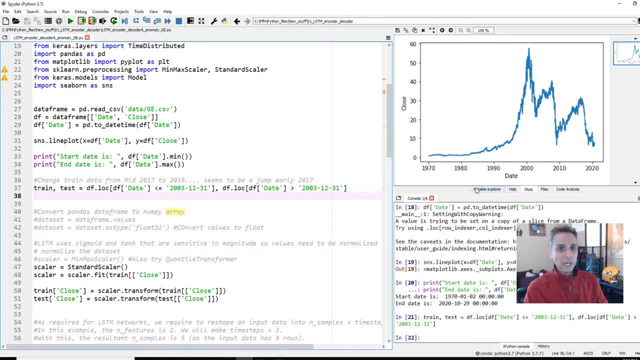 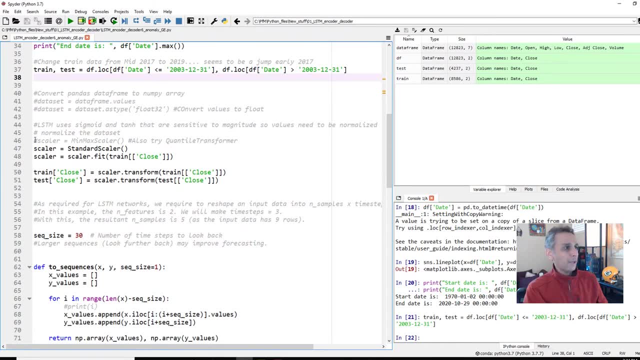 just show you the process, okay, so let's do that, do our training and testing. So now we have our train and test datasets And finally let's go ahead. You see how I was trying to do min max scalar. It doesn't make sense in this case. Let's. 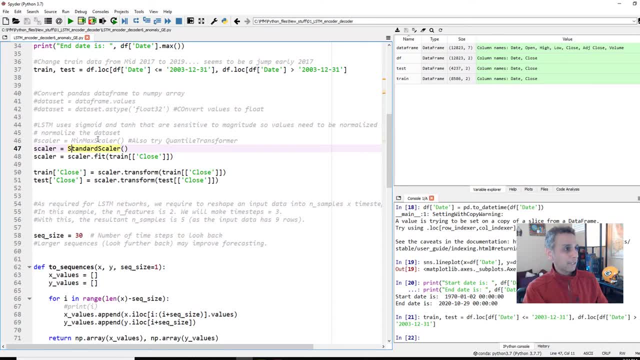 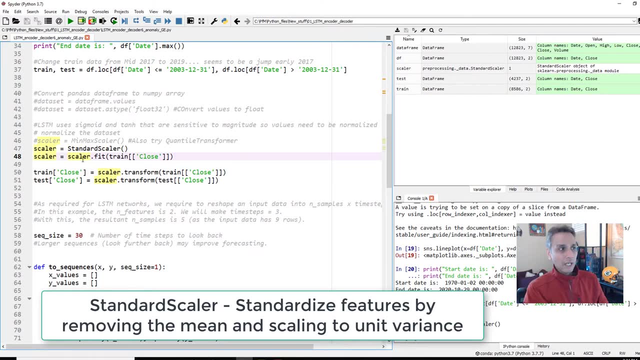 go ahead and do standard scalar, Okay, Which is just normalizing everything I think below between zero and one. So let's go ahead and do that. So we just defined our scalar. Now let's fit that scalar onto the training data and then apply that. Okay, So we fit this on the training data. 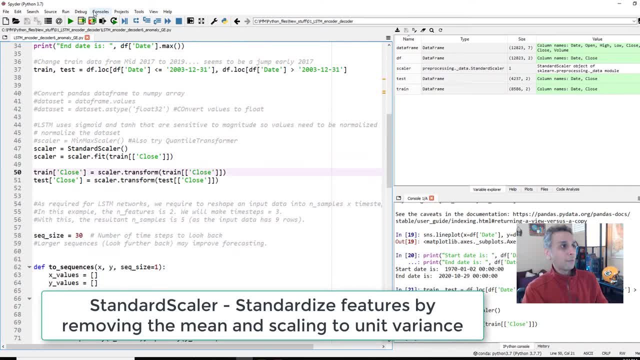 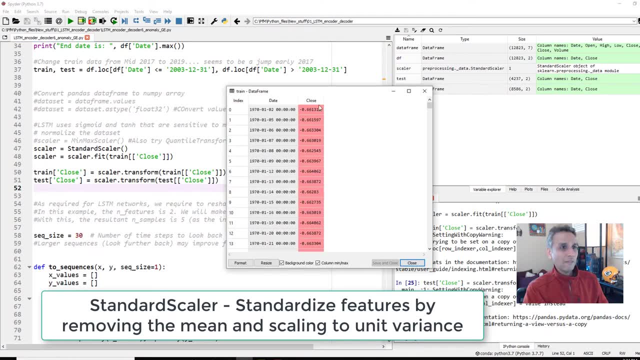 which means now we have a model that we can use to transform our both training data and testing data. Okay, So that's what we just did. Now, if I open my training data, you should see all the values to be: oh, it looks like it's a mean, is around zero and it distributes data between minus. 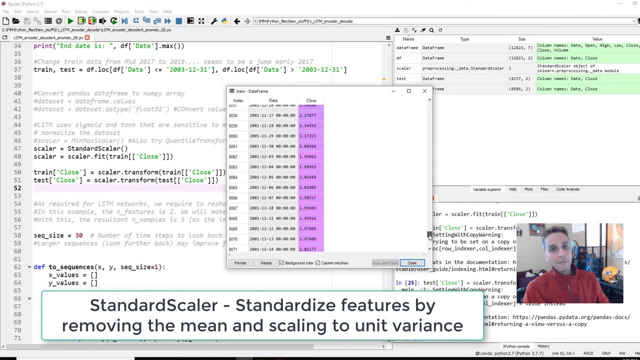 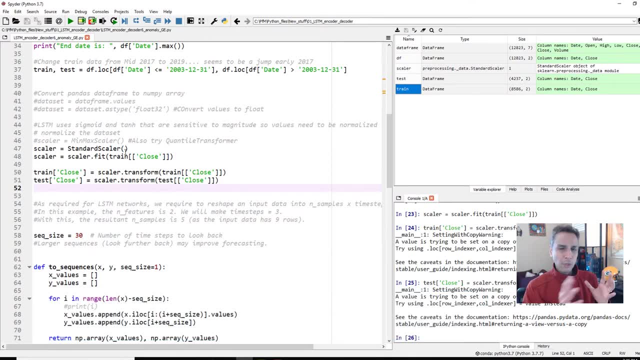 one to one, Not even minus one to one. I should have done my homework in terms of what standard scalar does. Min max scalar is basically: it looks at the minimum and maximum and squeezes everything to below zero and one, if I'm correct. Okay, So I'm using standard. 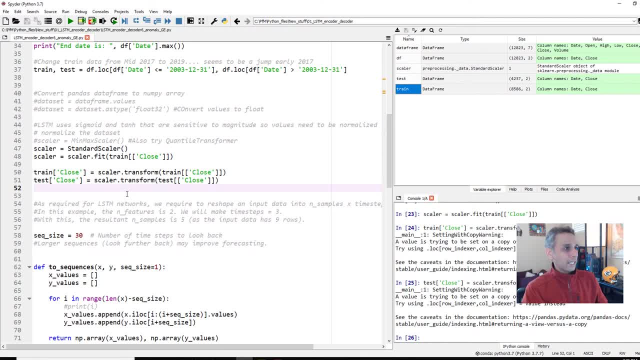 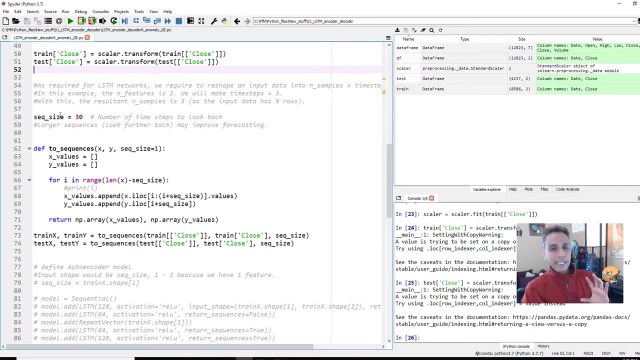 scalar, which works fine here And now let's actually look at. I mean, this is the stuff that we already did in a few of our previous videos when we looked at time series. So all we are trying to do is take our one long time series and break it down into different input sequences. 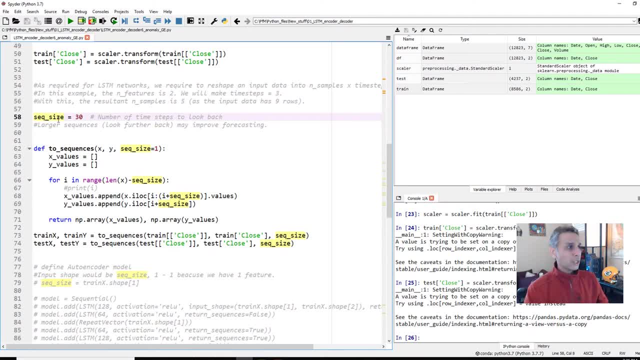 And you know, like X and Y values. So here I chose a sequence size of 30, because in the example I just I just showed you in the presentation, the sequence size was 30. Okay, So that's exactly. 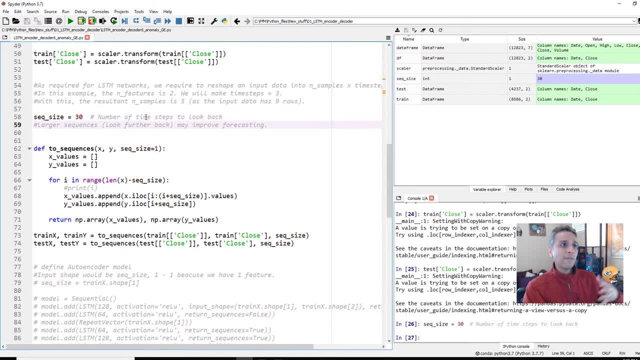 the same situation we are using here. What does that mean? It's basically number of time steps to look back and use that for our training. That's, that's what the sequence size is Okay, And the sequence size has an effect in terms of how the model gets trained, how accurate it is. 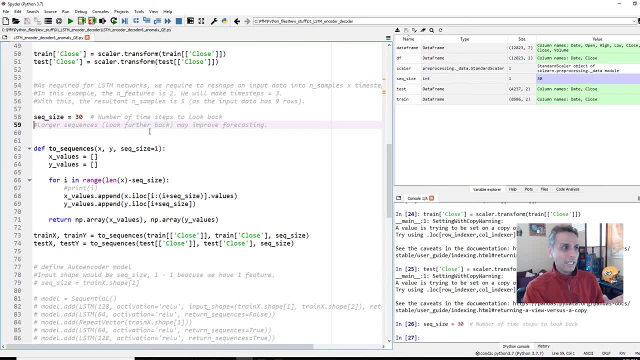 And it completely depends upon your data itself. Okay, So I'm just using 30 right here Now. this is the function we used quite a few times in the past. All this function does is it takes your- you know your- values. 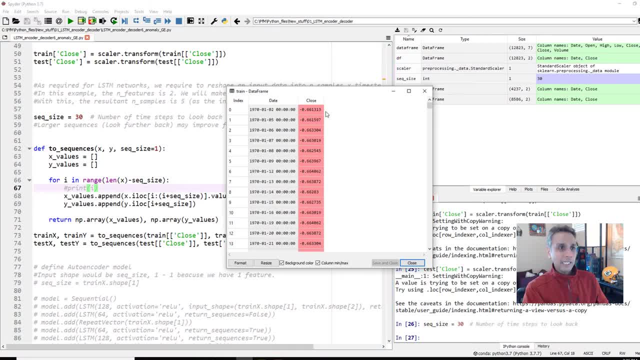 you know, in this case the training data right here. let's open this and see it takes your training data and it takes the first 30 as X and the 31st one as Y, and then it moves one down: Okay, The next 30 as X and the 32nd one right As your Y. 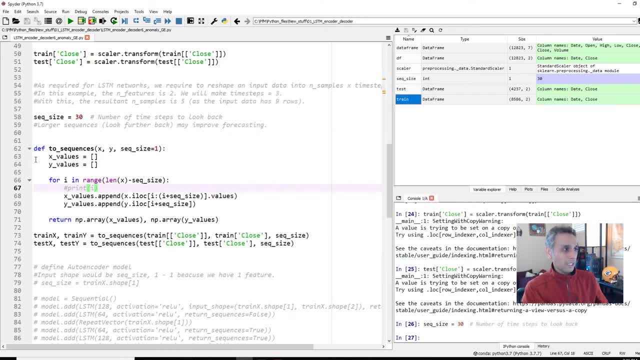 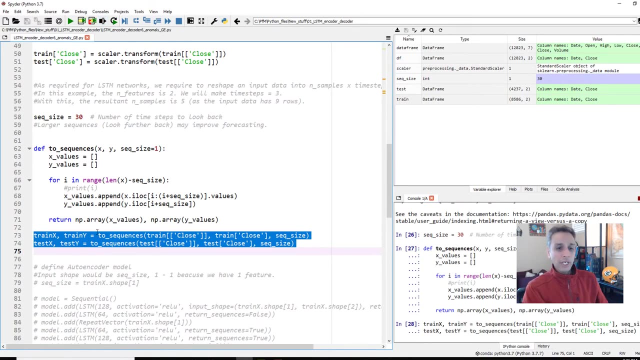 and so on. it creates these mini sequences. So that's exactly what this is doing. It's so let's go ahead and run this And now let's apply that to our training dataset and testing dataset that we just extracted. Okay, So let's go ahead and create our X and Y. All we're trying to do is 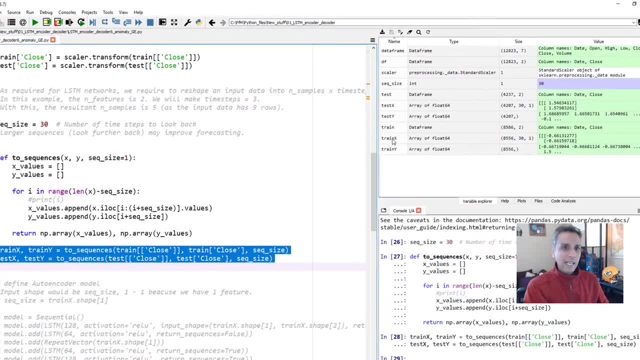 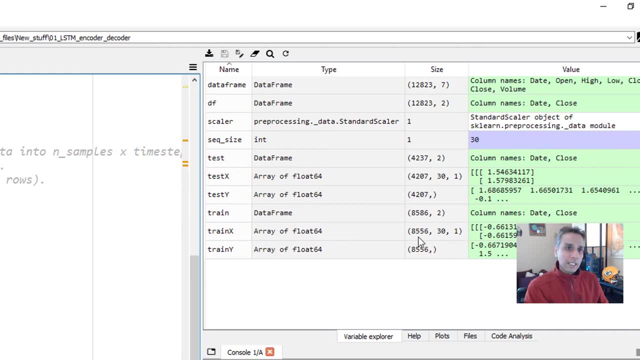 create X and Y And once this is done, you'll see that our train X has a size of 8,556.. Okay, By 30, by one, 8,556 was our train data. Okay, 8,586.. And now we have 8,556, because at 8,556, when you go 30, you reach 8,586. 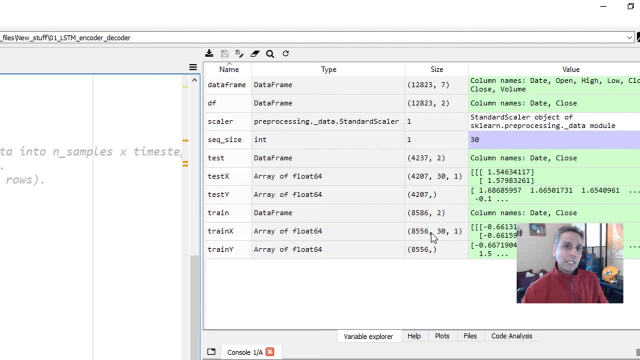 And after that there is no 30. So it stops there, Okay, So that's basically the operation right there. And then you have the train Y, which is basically what we are trying to fit this to. So, in other words, our X is the sequence, or Y is what comes next in the sequence, And the next is the. 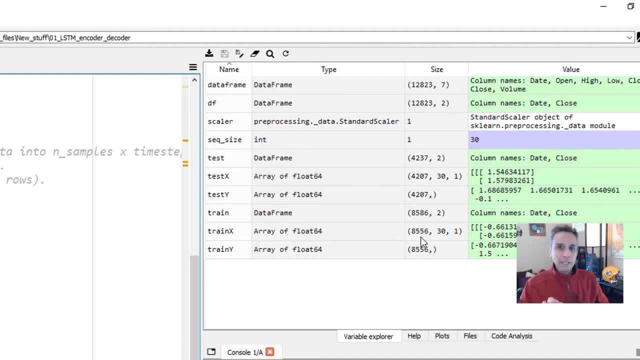 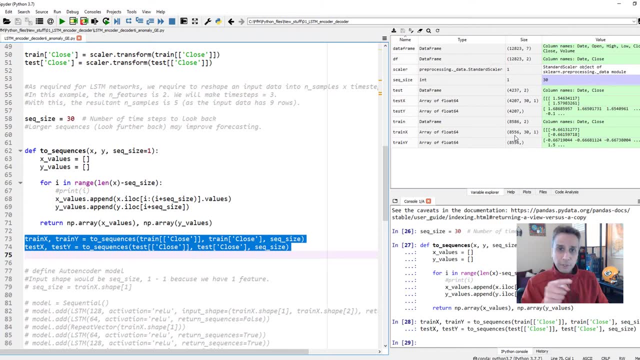 sequence continuing And our Y is the next sequence. We did exactly the same even when we did our natural language- not natural language, but when we did the text prediction sequence: what letter comes next? sequence: What letter comes next? Okay, Once you get this, everything else is pretty straightforward. 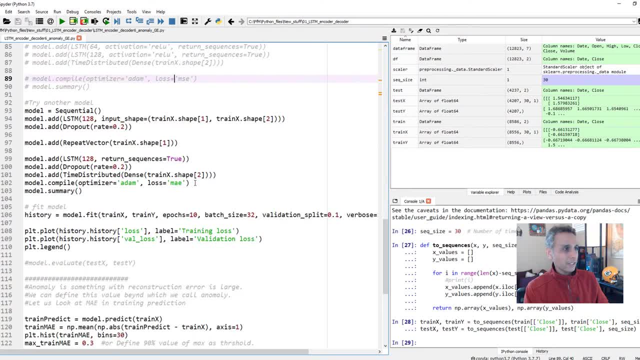 I was experimenting with a different model. You can always do that, And here is another model. So what I'm trying to do here is LSTM with 128 units, And then I introduced dropout Again. this is the regularization, So you're not overfitting Again. this is you can experiment. Okay, Originally I had 128, 64,. 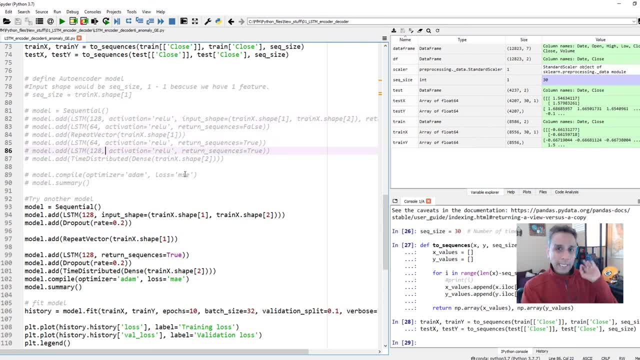 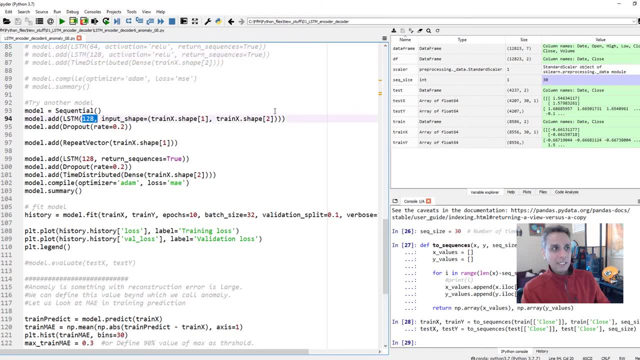 repeat vector 64,, 128, exactly the same thing I showed you in the presentation, but this one is working better, So I'm just going to show you this one. Okay, Which is one LSTM. That's it, Which means I'm not returning the sequences. Yeah, By default return sequence is false. And then I'm. 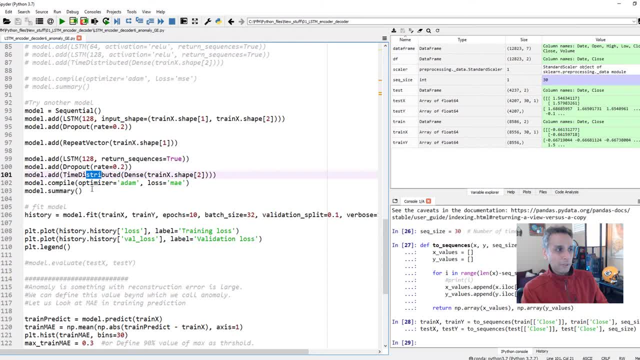 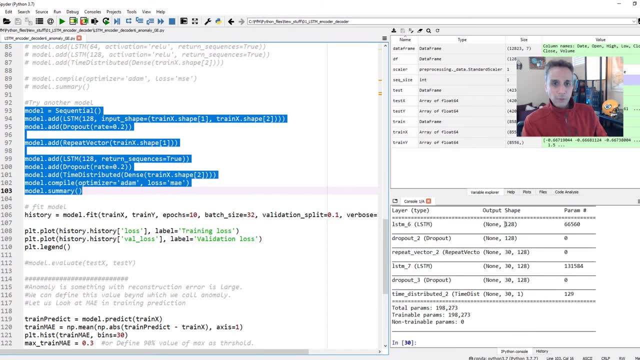 going to add repeat vector and then 128 and time distributed. That's pretty much it, Okay. So let's go ahead And print out the summary so you can have a quick look at what's going on. So 128,, 128,, 30 by 128,. 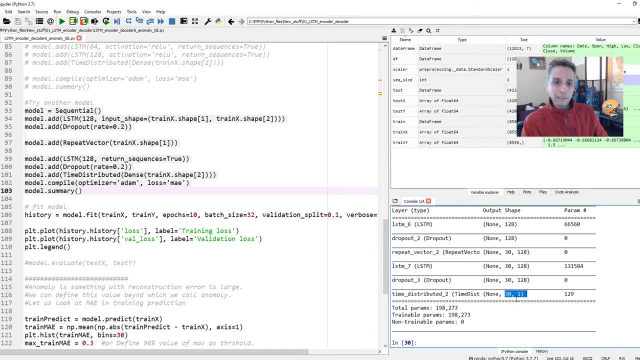 30 by 128. And finally, we're going to return a final. you know output would be 30 by one. Okay, Let's go ahead and train only for 10 epochs for this video, but maybe you need more epochs And. 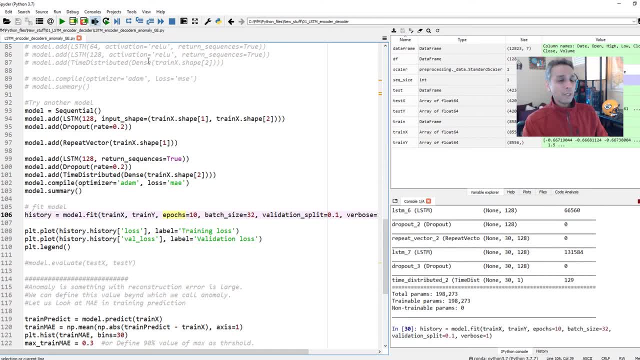 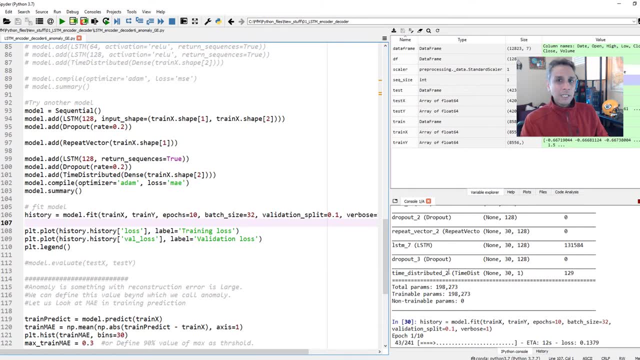 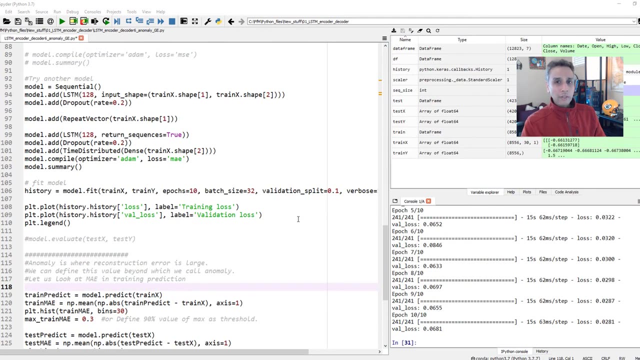 this is a bit slow, So let me pause the video and we can continue this. Even with this limited amount of data. this is a bit on the slow side, Okay, LSTMs are a bit slow, Okay, So let me pause and then continue as soon as this is done. Okay, So there. 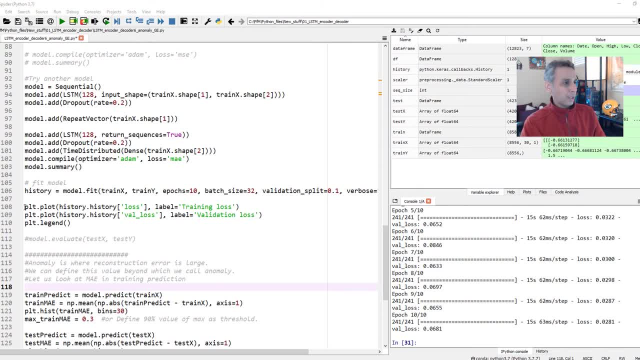 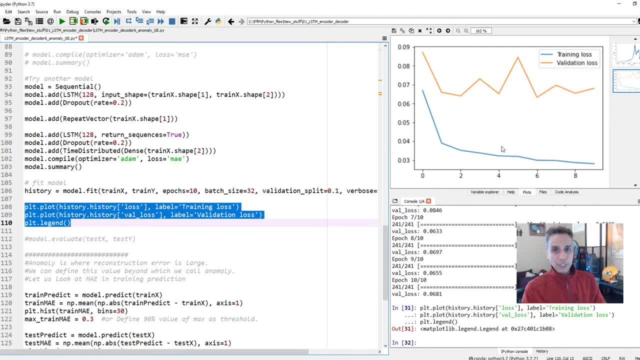 you go After a few minutes, it's finally done And let's see how the loss looks like. Okay, The loss curves. Let's go to our plot. Absolutely horrible, I bet, if you just go like 20,, 30 more. 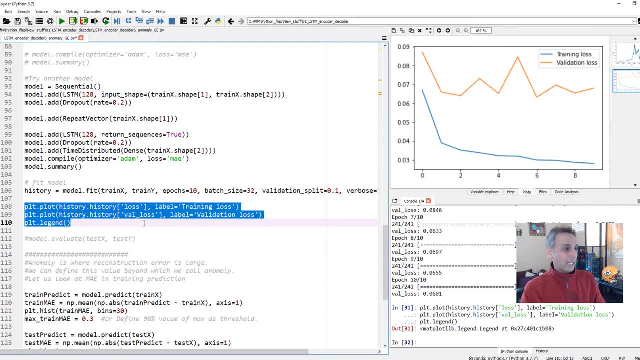 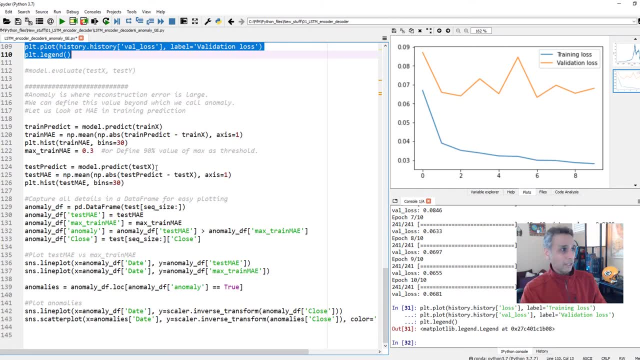 epochs. maybe there'll be some convergence here. Okay, So now let's go down and start looking at our mean absolute error or the construction error there. Okay, So how do we do that? Let's go ahead and predict on our training data. And again, you know how to do that: Modelpredict on our training data. And now let's. 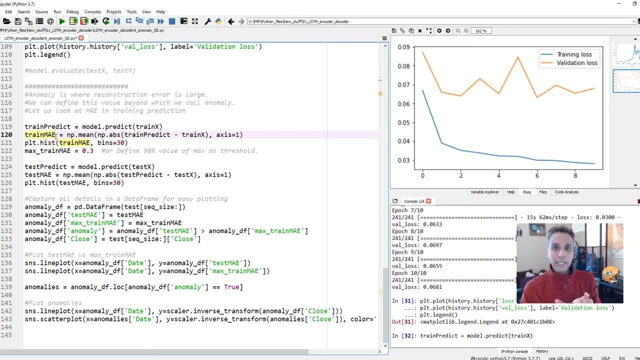 calculate the mean absolute error. What is the mean absolute error? You look at the error, take the absolute value and take the mean of these. So basically, we are doing the mean of the absolute of the error. This is as straightforward as it gets Train predict, which is the prediction right now. 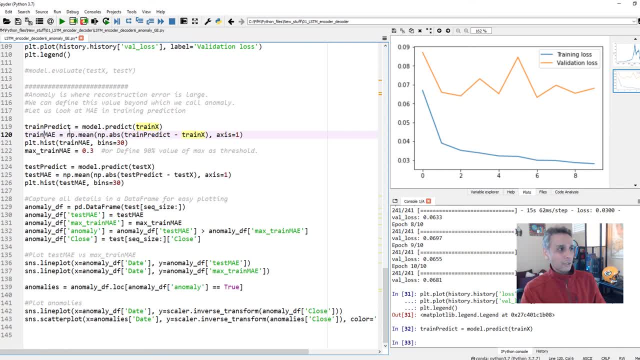 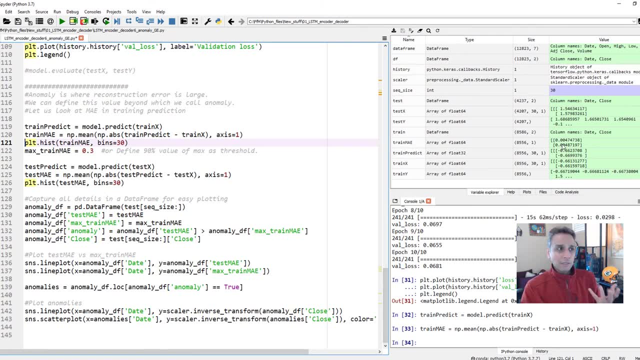 is train X, which is our actual values, And you're just going to calculate the mean absolute error. And if I go back here, train MAE, it's giving me some values, but I don't know what that means. Okay, So let's go ahead and plot it. Plot the mean absolute error values for all of our X values. 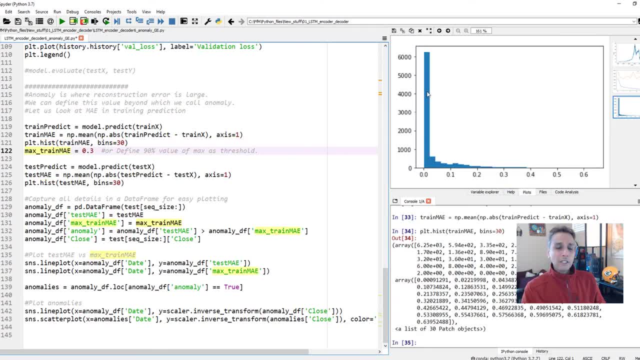 right, Or train values, Sorry. So let's go ahead and plot And it looks like the lot of mean absolute error is a 0.00, something right here, And it's actually going up All the way to maybe even 0.6, right there. Okay, So one way to actually define the threshold value. 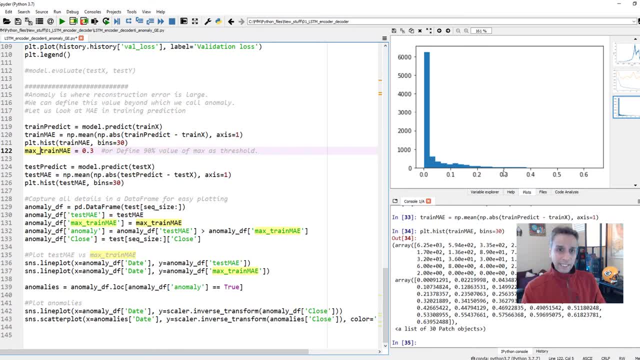 or the maximum value where it's acceptable is just look at the maximum and say, okay, the maximum is your threshold value beyond which. So when new data comes in, if the error is above 0.6, then that's an anomaly, Okay, And the other way you can do is: okay, I'm not really comfortable with 0.6.. 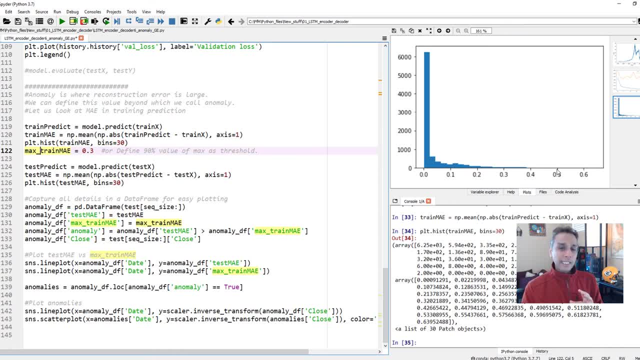 Let's just say 90%, Okay. So let's say 90% of that value, okay is probably the threshold. So it's up to you. what is the threshold value? I just define something as 0.3 because I see bulk of the data is right here and 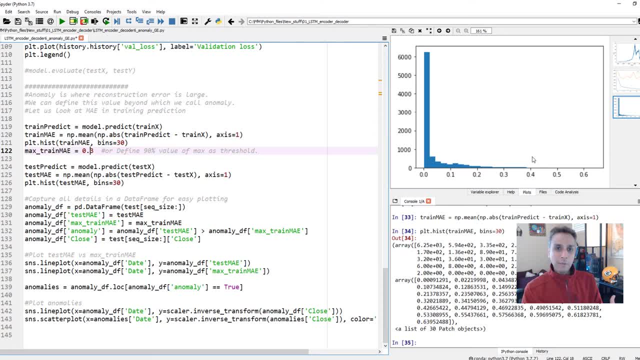 everything above 0.3 is probably, in my view, considered as anomaly that I can go back and have a look at what's going on during that time. Okay, So I just defined a value of 0.3, hard-coded this to 0.3, but it's up to you, like I just said. So now that we have a threshold value, 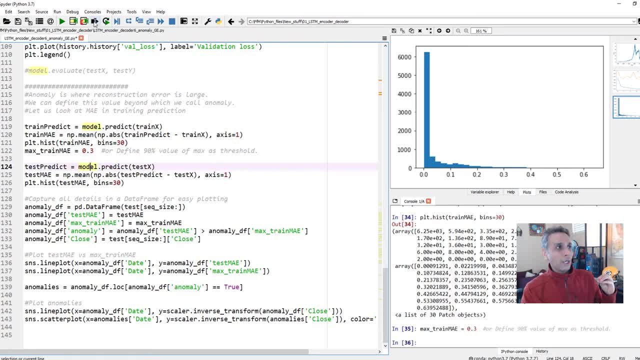 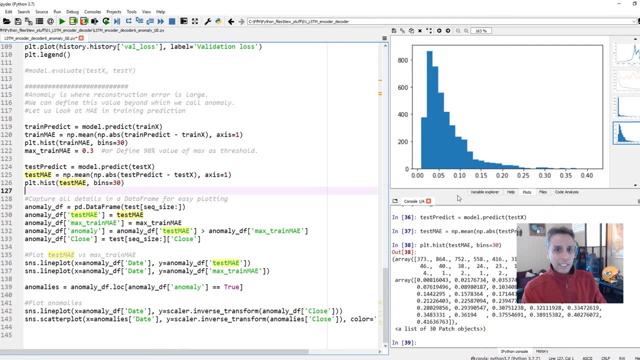 now let's go back to our test data and then let's go ahead and predict the test, Okay, And let's do exactly the mean absolute error for test and let's also look at the histogram for test. Oh, our test data is actually fitting much better, You see. the maximum mean absolute error is like 0.4.. So if I 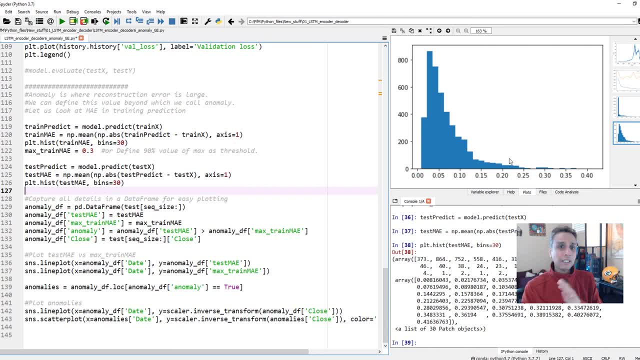 set my threshold to about 0.6, then in my test data, nothing is anomaly. Yeah, Even down to 0.4, nothing is anomaly. So I set it to 0.3.. So we should see some anomaly data points, Okay, In our original data. So this is just our again. 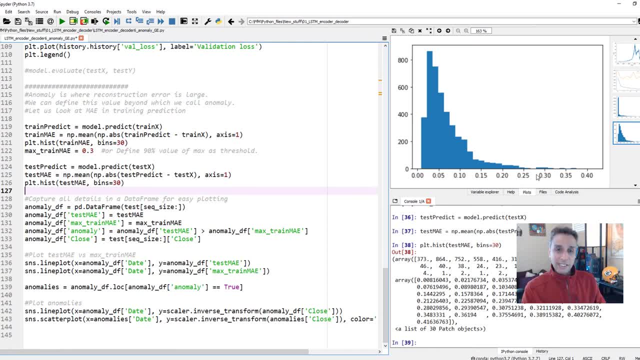 reconstruction error or mean absolute error, if you want to call this in this case where we are picking this threshold value. Okay, So now let's actually capture the anomaly. Now I'm going to go back to the original data and say, okay, is this above or below? Okay, So how am I? 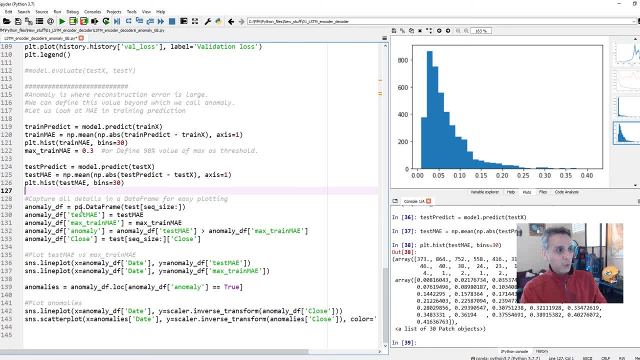 doing that, I'm going to capture all the details in a data frame. So I'll create a data frame for test sequences. Okay, I'm only looking at a test right now And I call that anomaly DF data frame. Okay, And now I'm capturing all my test mean absolute error. 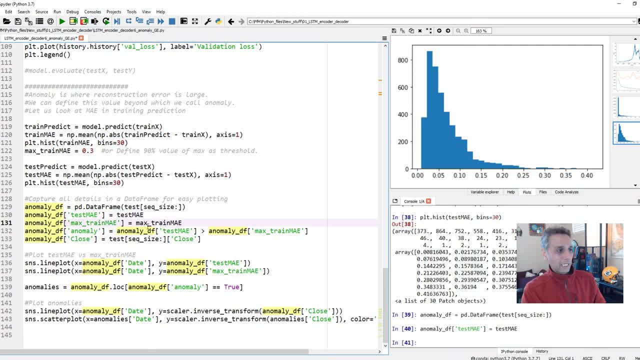 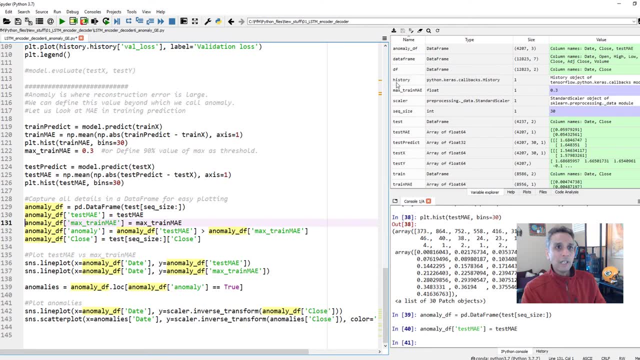 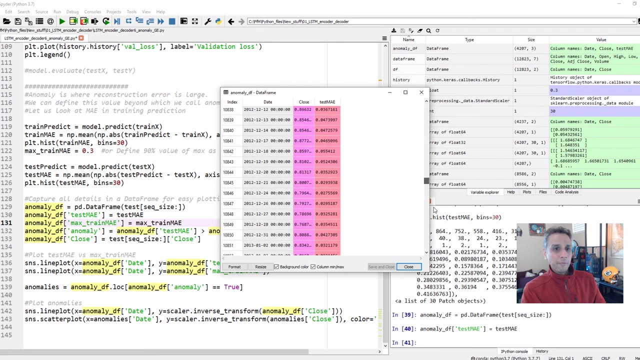 as part of that. And then max stream MAE is basically 0.3 in this case. Okay, Let's open it so we can see this in a progressive way rather than just me talking about it every time. So there you go. So we have all of these data points. Okay, That are part of our test data set. And then here: 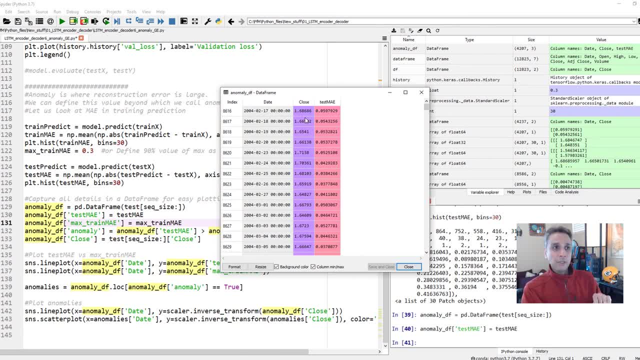 is the closing value, And here is the test data set. And here is the closing value And here is the mean absolute error corresponding to that value. All we are trying to do is now add what the threshold is and just see: is this above or below? That's pretty much it, Okay. So that's exactly what. 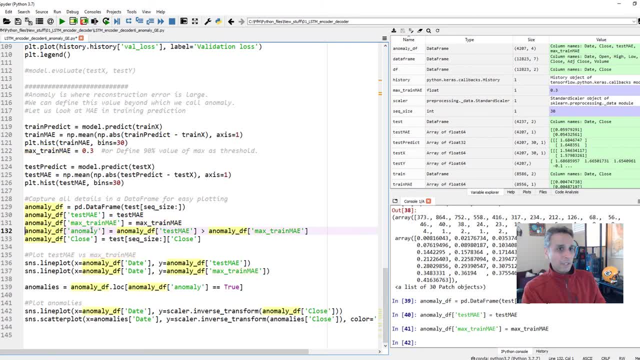 we are doing now, Add this. And now I'm saying, okay, let's open this one more time. So you can see, now I added 0.3.. There are many ways to do this And this is one way I chose to do. And now, 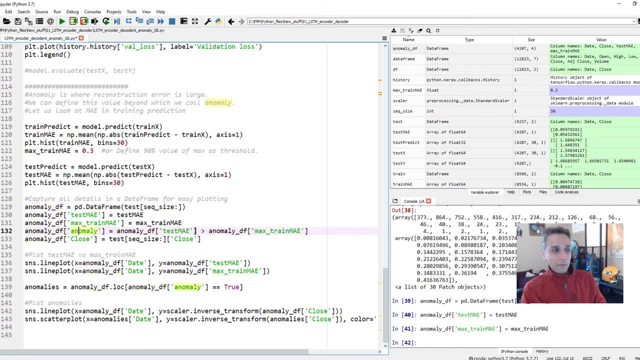 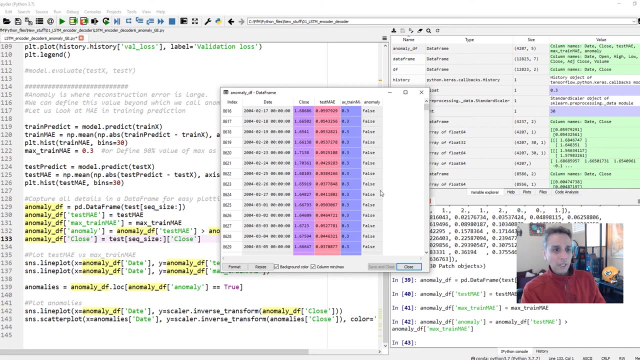 I'm going to add another column, which is going to be a Boolean column, saying: is this a greater or greater than you know, this value, or is it less than right, True or false? So let's go ahead and open this again, And now you should see, these are all not anomalies, you know, or is it anomaly, or? 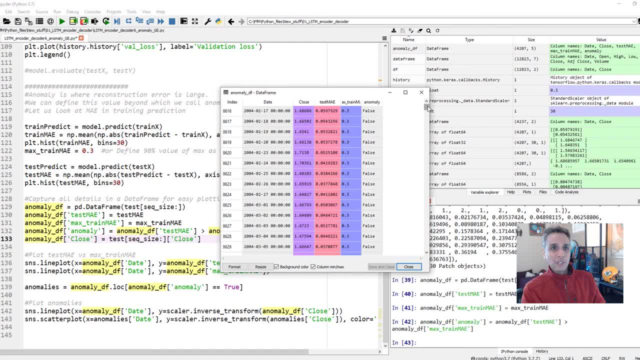 is it not an anomaly? right So 0.3, this is 0.05.. So it's not an anomaly. I'm not even sure if there are any trues in this case. Let's keep going down. Maybe we have to plot train to see the anomalies. 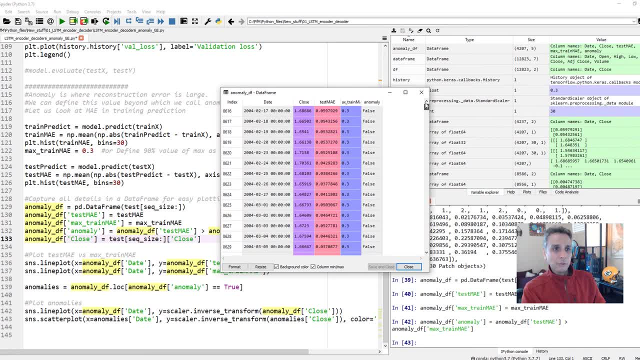 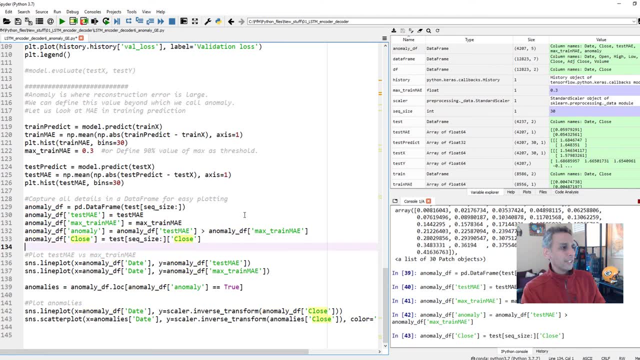 In the test data. not much going on. I'm pretty sure there's got to be one or two, but okay, That's okay. So now let's go ahead and finish this off. Anomaly close is: let's go ahead and. 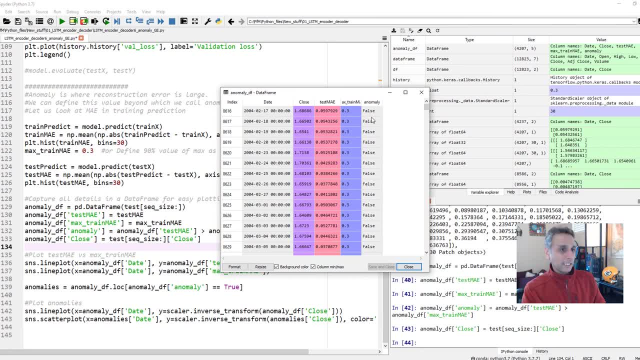 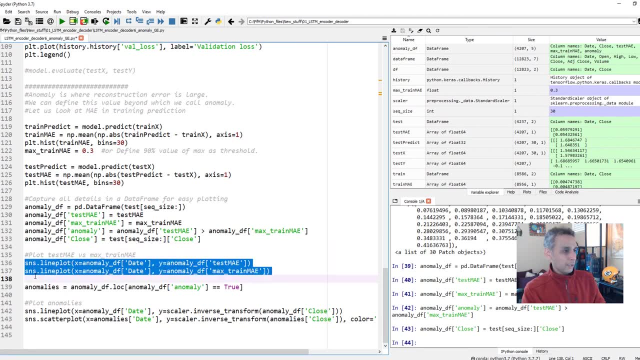 look at our anomaly right there, And now let's plot it, Okay. So I think this is the best way. I was trying to explain something using the values over there. Plotting is always the best thing. So let's go ahead and look at the plot right there. So here you see all the data, right. 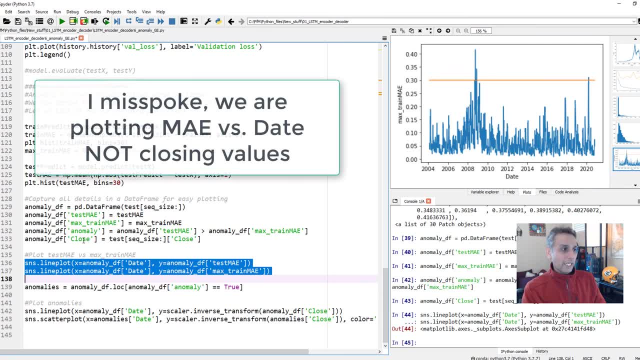 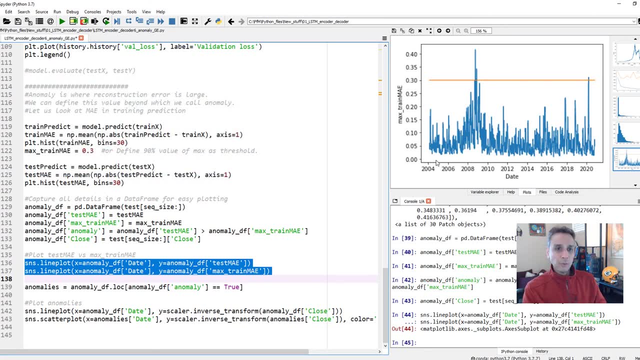 here. So all I'm trying to do is plot the closing values in our test data set And remember our test data set starts somewhere around 2000,. actually 2004,, because up to 2003, it was training data set. So from 2004,, all the way up to here, there are only a few data points right there that are 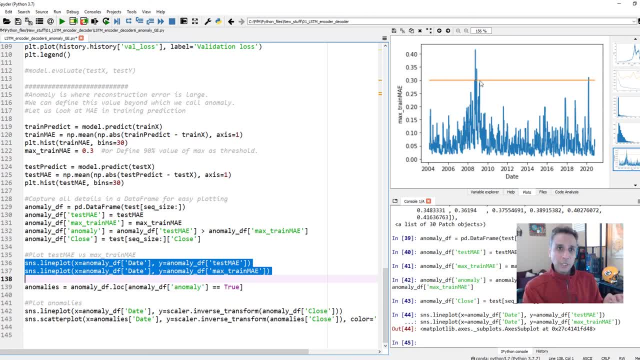 above the reconstruction error that we set as threshold, which is 0.3.. So I'm just plotting this horizontal line as the threshold. So that's it. So now we are looking at this space where we have date versus maximum, you know, or this. 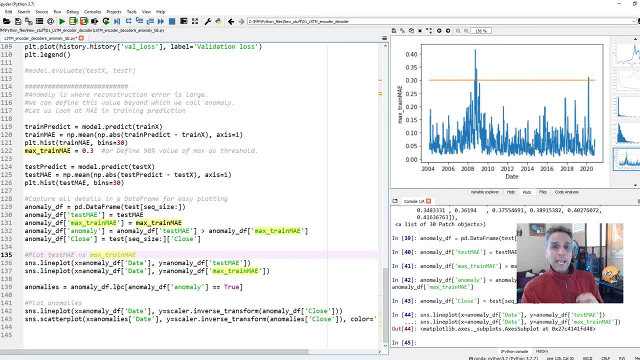 mean absolute error, but then let's actually extract the anomalies for the original data. So, basically, my anomalies data frame is everything where my anomaly equals to true. So let's go ahead and do that. And now let's go ahead and plot, Okay. 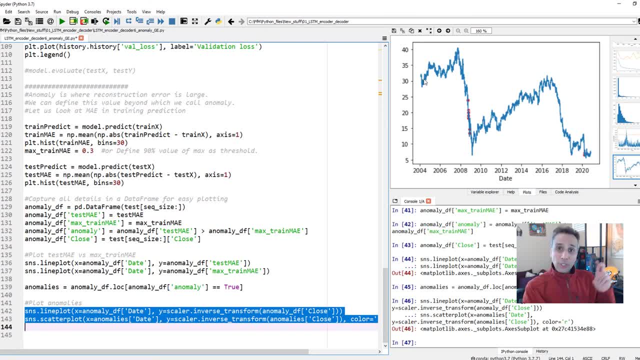 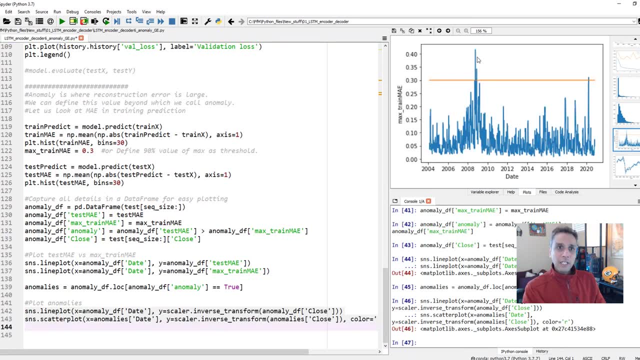 And there you go. So now looking at this data, the original data, Okay, So now we are looking at this data. So now we are looking at this data. So now we are looking at this data. So now we are nothing, nothing, nothing. and here you see the peak, right here. these values, they 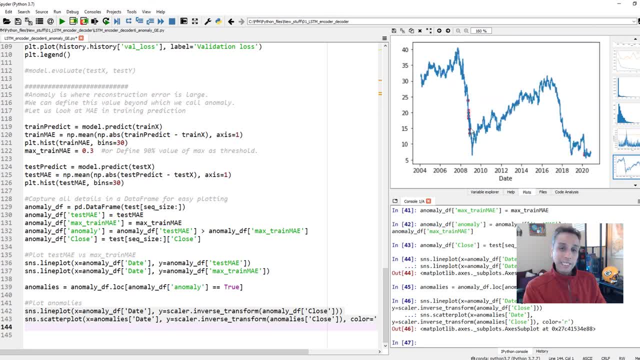 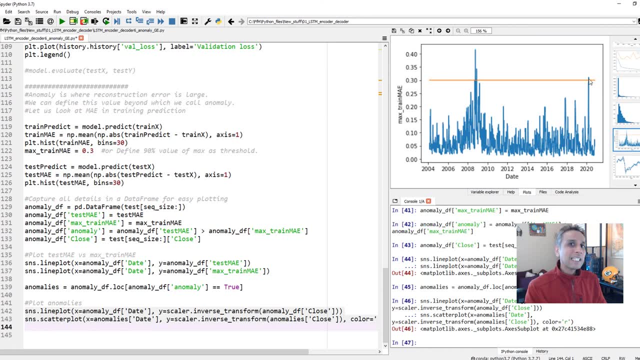 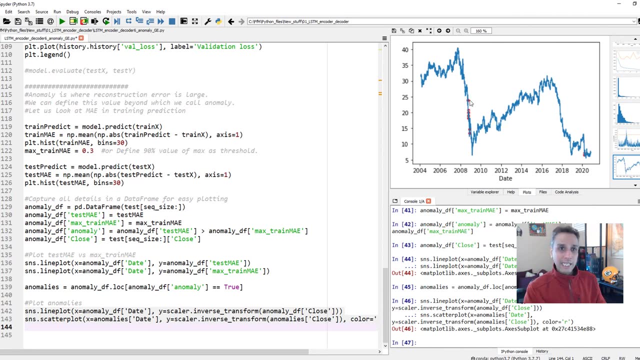 apparently correspond to these and these are the anomaly days, and apparently we also have something right near 2020 right around there. maybe it corresponds to this little thing right there. okay, so that's what these anomalies correspond to. so now you can go back to these days and I and then see why there is an 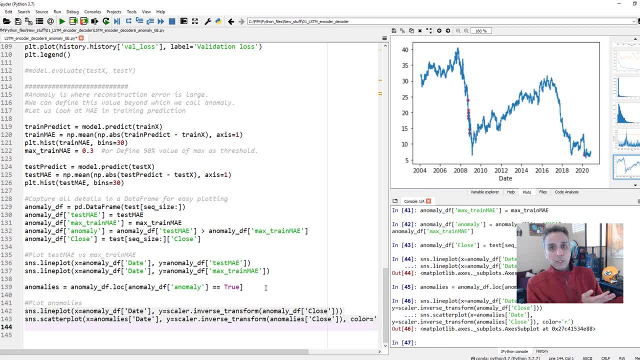 anomaly. okay, and what does that anomaly mean? this system doesn't know what an anomaly means. obviously it's looking at the training data, looking at the reconstruction error. a good thing, would I mean. I think the best thing to do. I was just thinking about this out loud. you used to use plotly to plot these and 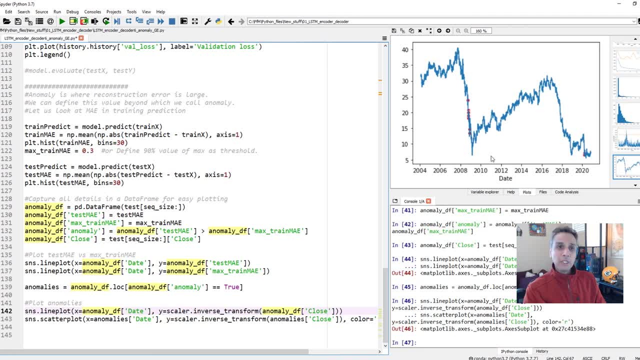 then wherever there is an anomaly, it would be nice to actually have the news feed from that day tagged as the hover over, so when you put your mouse over this it kind of tells you the news for that day. then probably you can get some information about what happened that day to GE, where. 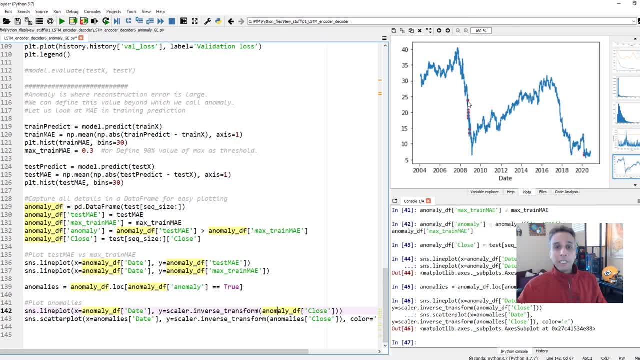 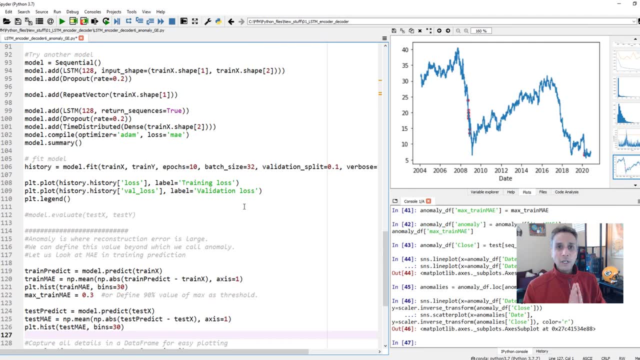 we are actually seeing this anomaly. okay, or not just GE, but the market conditions in general, but maybe specifically to GE. so I hope you learned something new here and again. all we are trying to do is stack these LSTMs into our encoder and decoder and then train them and look at the- you know, reconstruction error in. 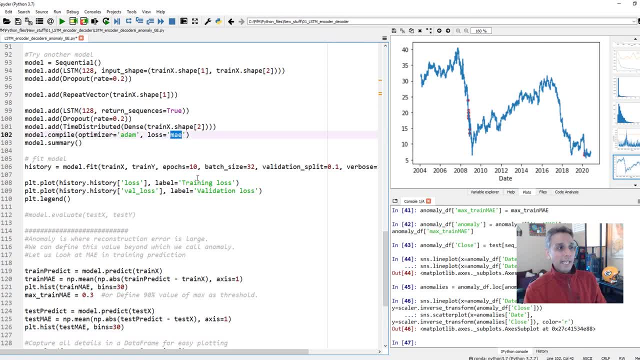 this case, we used MAE right as our last function and we are just looking at the mean absolute error, and anything above threshold is an anomaly. that's pretty much it, okay. so thank you very much and again, subscribe to my channel, because I am going to create cool videos for you and more.